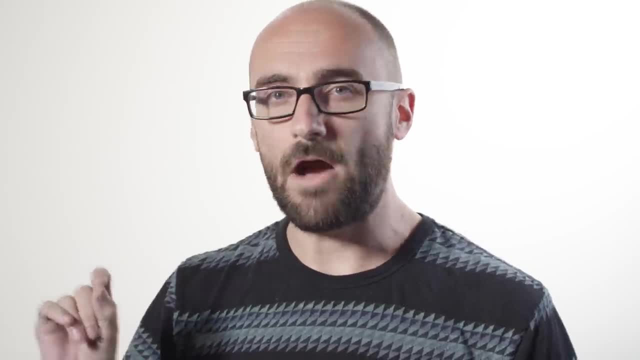 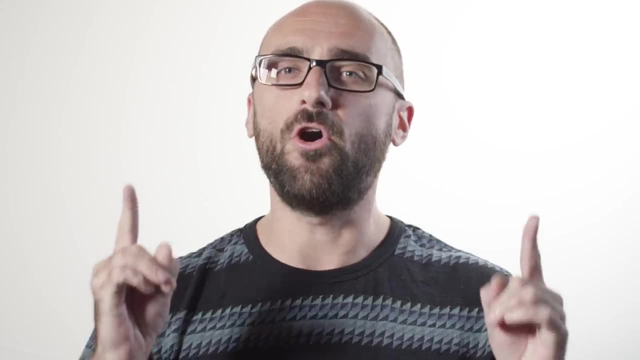 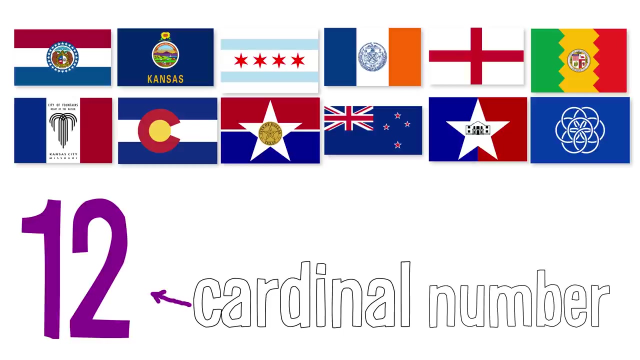 others. Let's visit some of them and count past them. First things first. when a number refers to how many things there are, it is called a cardinal number. For example, four bananas, Twelve flags, Twenty dots, Twenty is the cardinality. 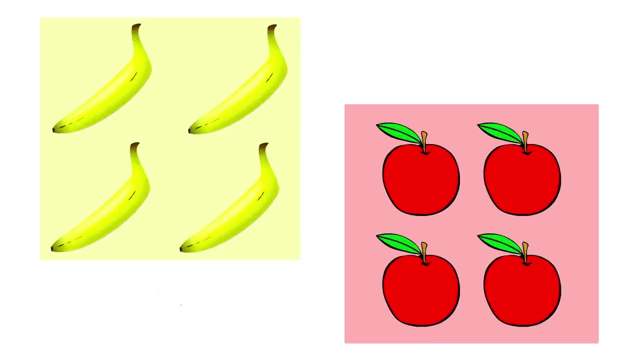 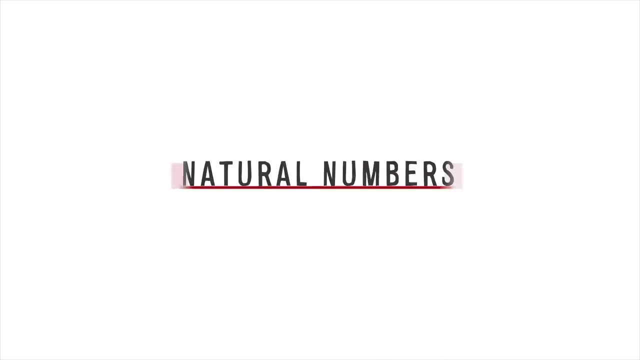 set of dots. Now two sets have the same cardinality when they contain the same number of things. We can demonstrate this equality by pairing each member of one set one to one with each member of the other. Same cardinality, pretty simple. We use the natural numbers, that is. 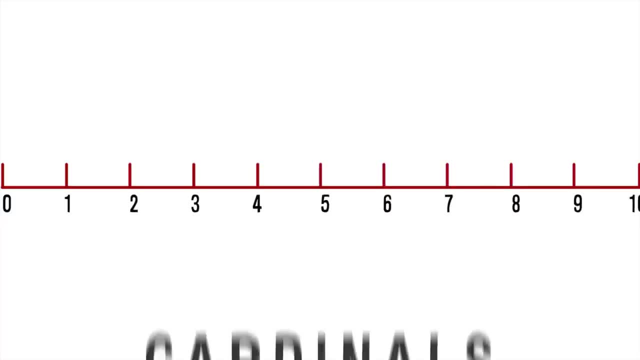 0,, 1,, 2,, 3,, 4,, 5, and so on, as cardinals, whenever we talk about how many things there are, But how many natural numbers are there? It can't be some number in the naturals because 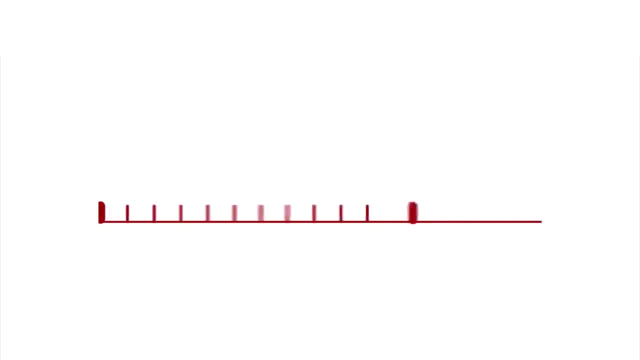 there'd always be one plus that number after it. Instead, there's a unique name for this amount: Aleph-Nol. Aleph is the first letter of the Hebrew alphabet and Aleph-Nol is the first, smallest infinity. It's how many natural numbers there are. It's also how many even. 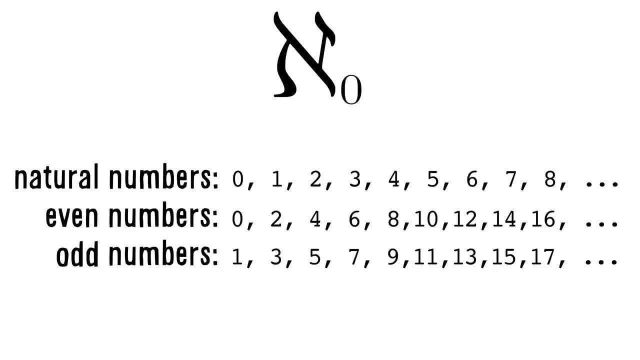 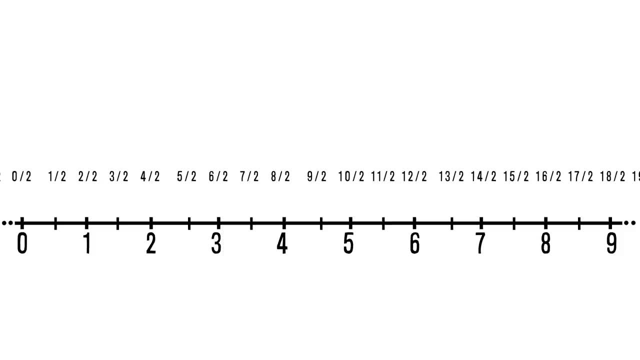 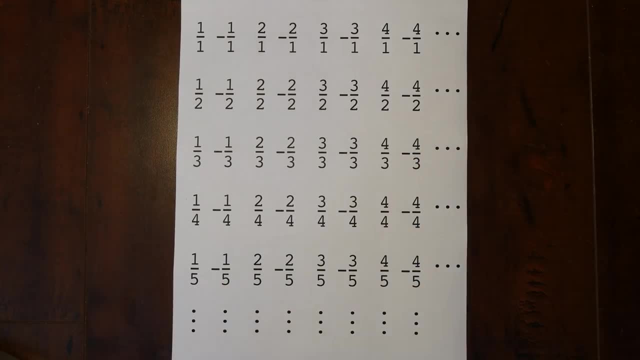 numbers there are, How many odd numbers there are. It's also how many rational numbers, that is, fractions, there are. That may sound surprising, since fractions appear more numerous on the number line, but, as Cantor showed, there's a way to arrange every single possible rational. 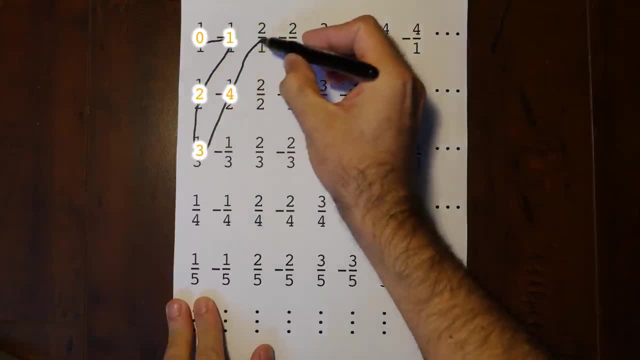 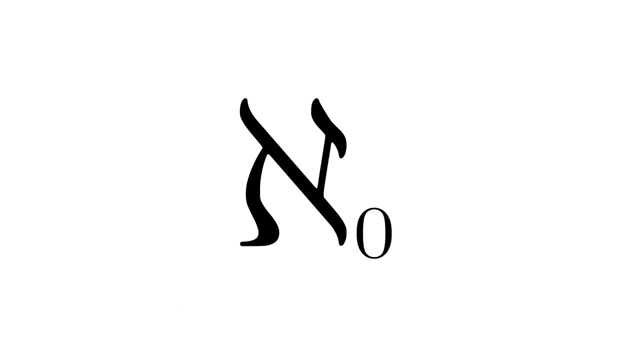 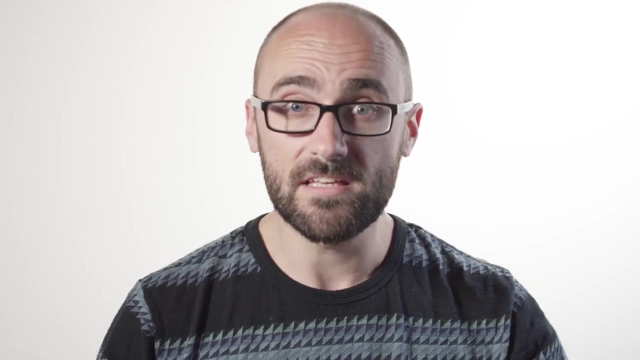 such that the naturals can be put into a one to one correspondence with it. They have the same cardinality Point is: Aleph-Nol is a big amount, Bigger than any other number, Bigger than any finite amount. A googol, A googolplex, A googolplex factorial to the 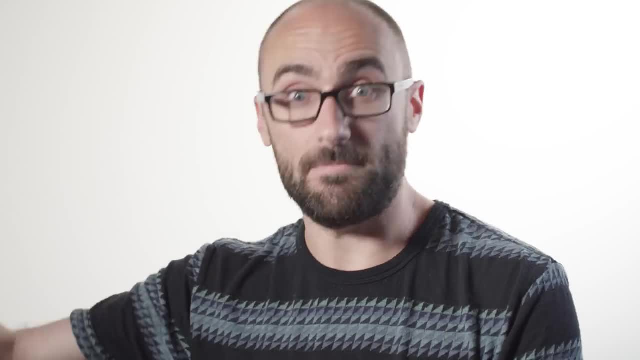 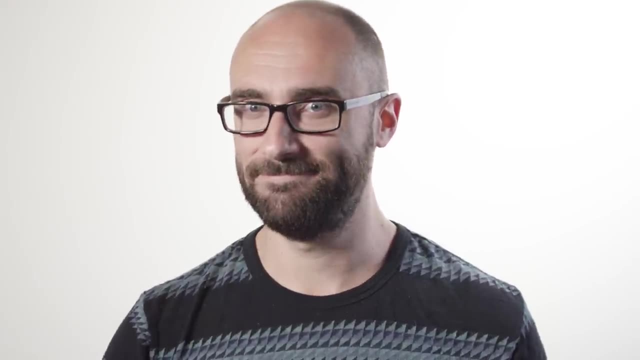 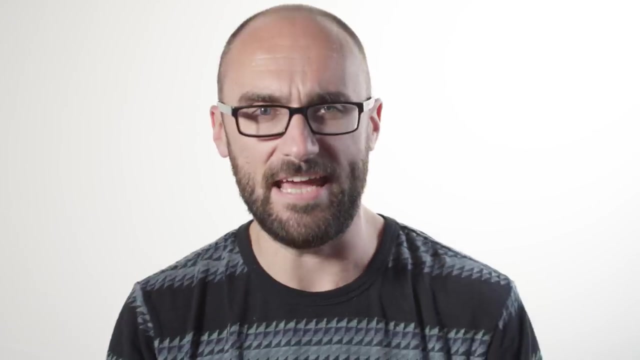 power of a googolplex to a googolplex. squared times Gram's number Aleph-Nol is bigger, But we can count past it. How Well? let's use our old friend, the super task. If we draw a bunch of lines and make each next line a fraction of the size and a fraction of the 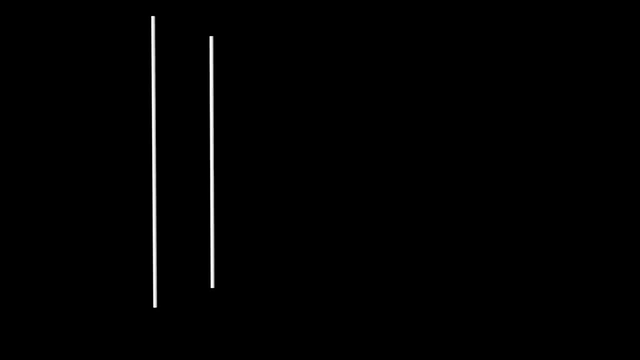 distance from each last line. well, we can fit an unending number of lines into a finite space. The number of lines here is equal to the number of natural numbers that there are. The two can be matched one to one. There's always a next natural, but there's also always. 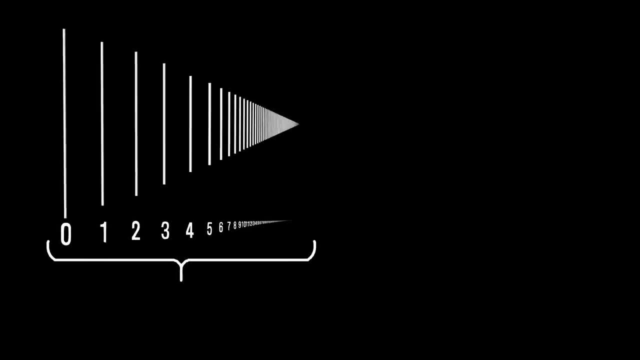 a next line. Both sets have the cardinality Aleph-Nol. But what happens when I do this? Now, How many lines are there Aleph-Nol plus one? No, Unending amounts aren't like finite amounts. There are still only Aleph-Nol lines here, because I can match the naturals one to one. 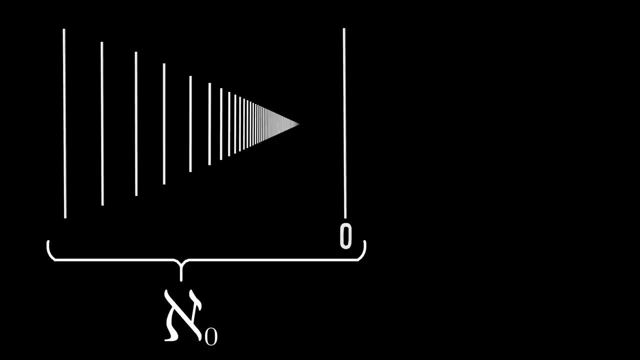 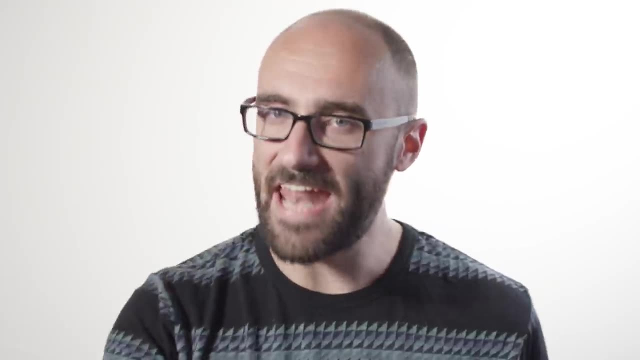 just like before. I just start here and then continue from the beginning. Clearly, the amount of lines hasn't changed. I can even add two more lines, Three more, Four more. I always end up with only Aleph-Nol things. I can even add another infinite Aleph-Nol of lines and still not change the quantity. 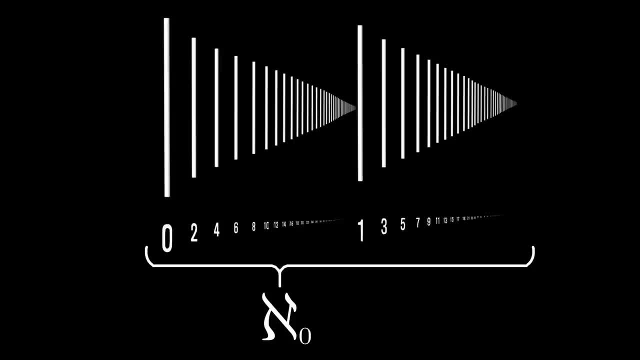 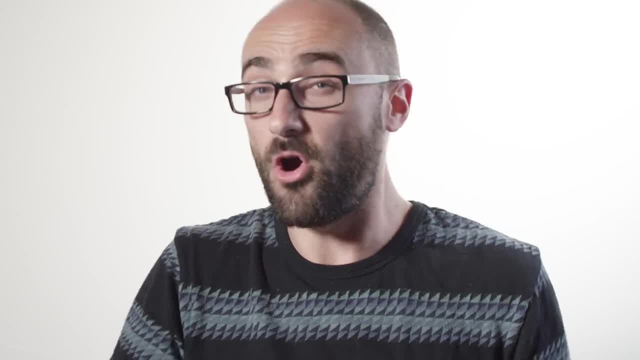 Every even number can pair with these and every odd number with these. There is still a line for every natural. Another cool way to see that these lines don't add to the total is to show that you can make this same sequence without drawing new lines at all. Just take: 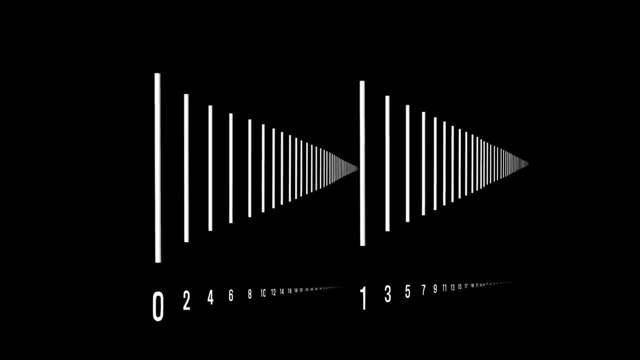 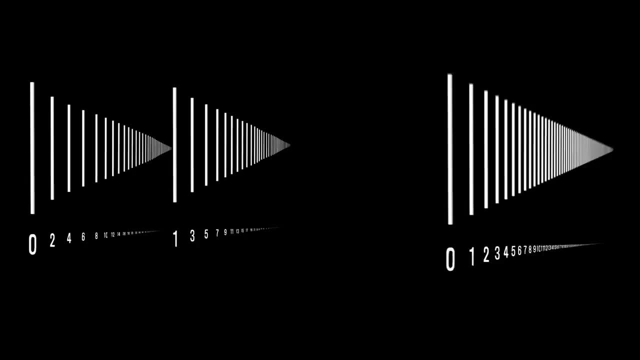 every other line and move them all together to the end. It's the same thing. But hold on a second. This and this may have the same number of things in them, but clearly there's something different about them, right? I mean, if it's not how many things they're. 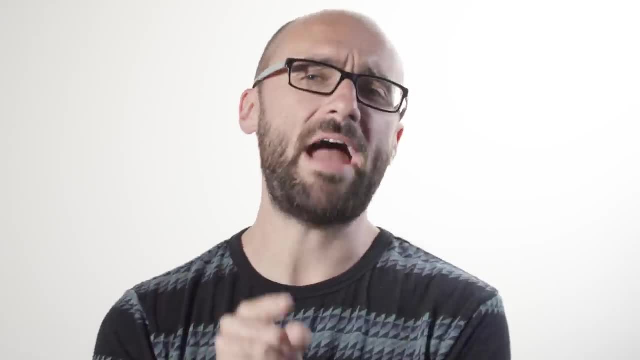 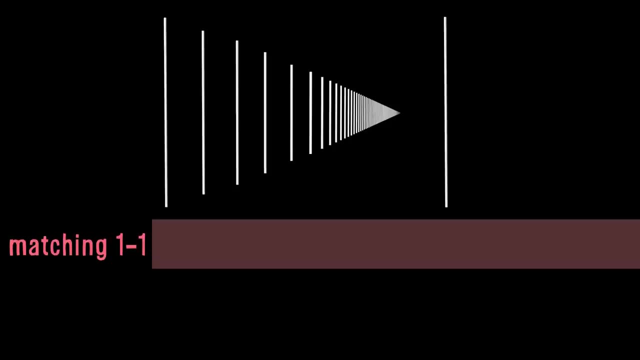 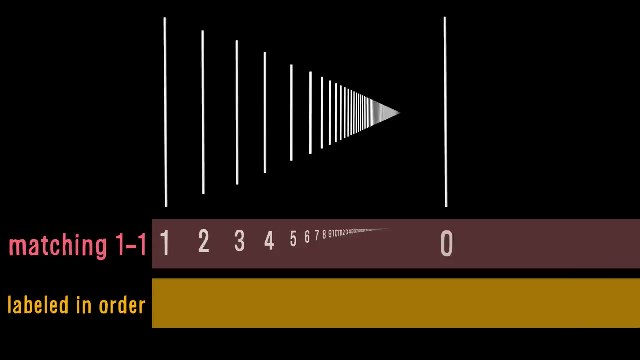 made of. what is it? Well, let's go back to having just one line after an Aleph-Nol sized collection. What if, instead of matching the naturals one to one, we insist on numbering each line according to the order it was drawn in? 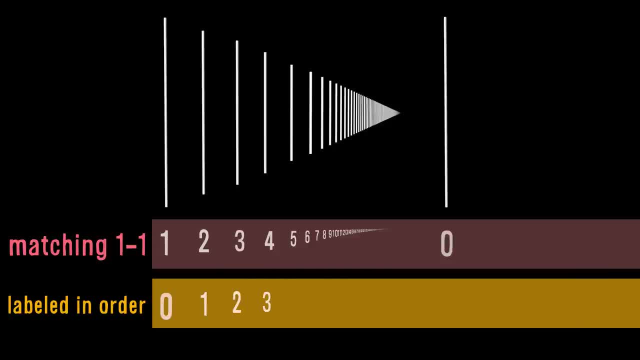 So we have to start here And number left to right. Now, what number does this line get In the realm of the infinite? labeling things in order is pretty different than counting them. You see, this line doesn't contribute to the total, but in order to label it according to the order it appeared. 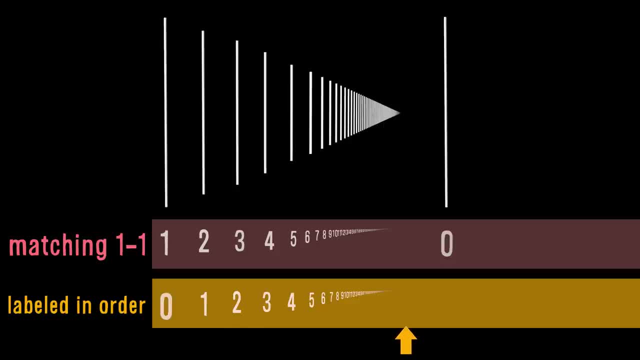 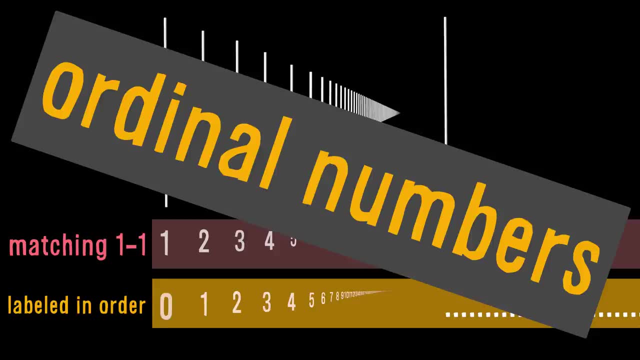 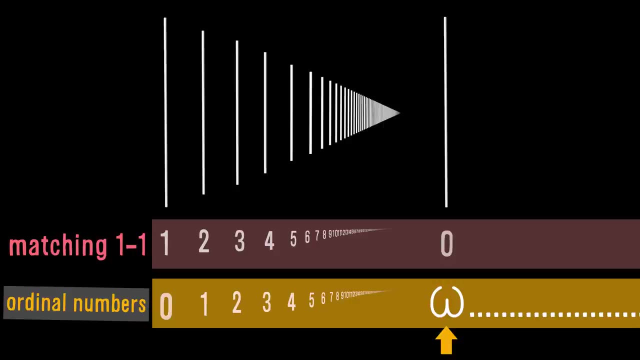 in. well, we need a set of labels, of numbers that extends past the naturals. We need order numbers. The first transfinite ordinal is omega, the lowercase greek letter omega. This isn't a joke or a trick. it's literally just the next label you'll need after using 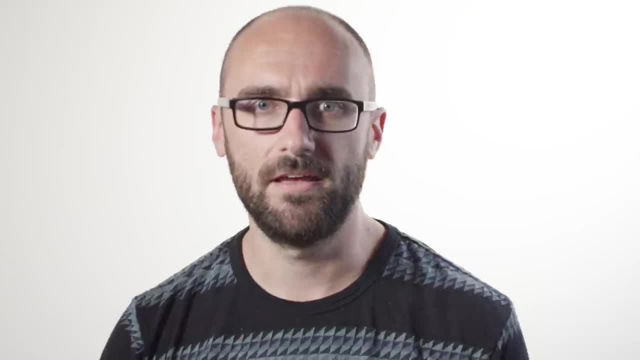 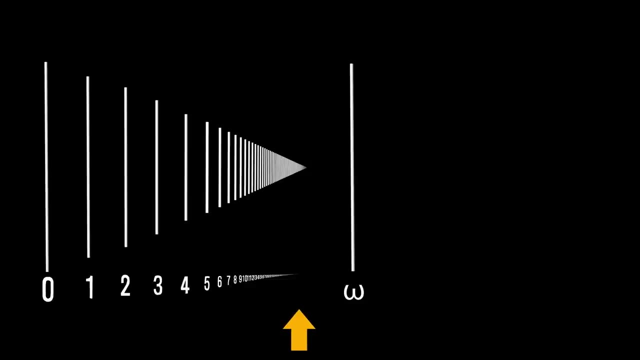 up the infinite collection of every single counting number. first, If you got omegeth place in a race, that would mean that an infinite number of people finished the race. and then you did. After omega comes omega plus one. This is a very simple way to label. 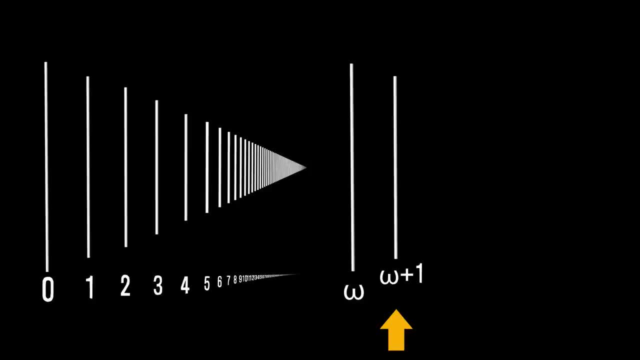 which doesn't really look like a number, but it is just like 2 or 12 or 800.. Then comes omega plus 2, omega plus 3.. Ordinal numbers label things in order. Ordinals aren't about how many things there are. 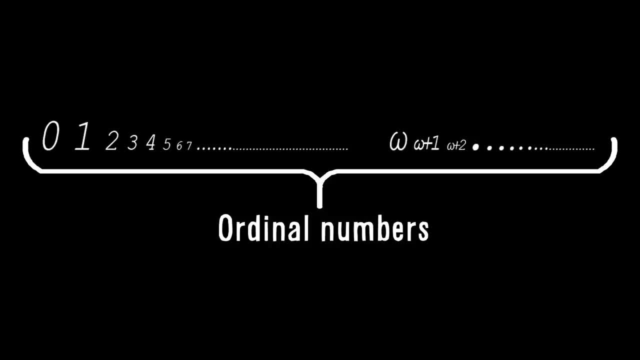 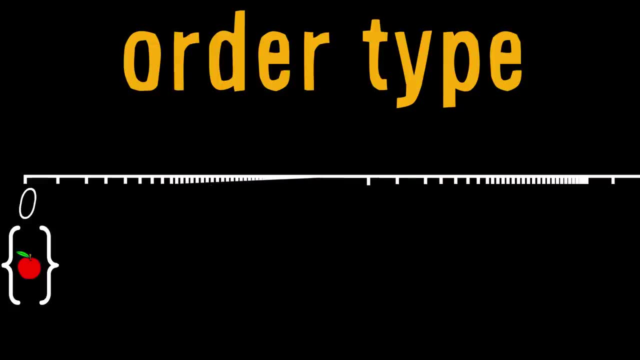 Instead they tell us how those things are arranged, their order type. The order type of a set is just the first ordinal number not needed to label everything in the set in order. So for finite numbers cardinality and order type are the same. 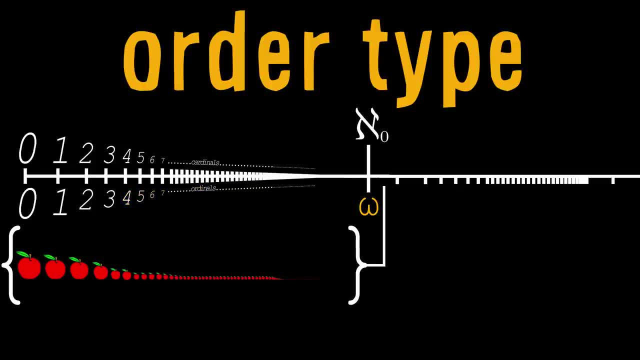 The order type of all the naturals is omega. The order type of this sequence is omega plus 1, and now it's omega plus 2.. No matter how long an arrangement becomes, as long as it's well-ordered, as long as every part is well-ordered. 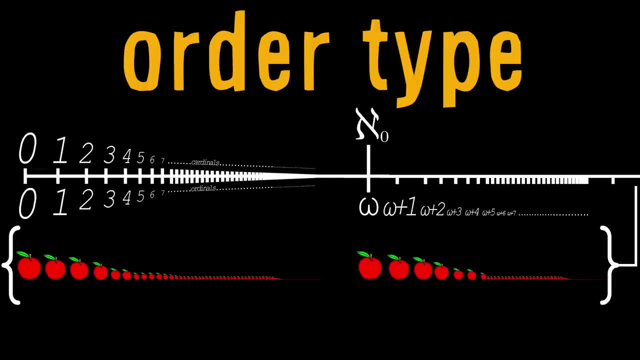 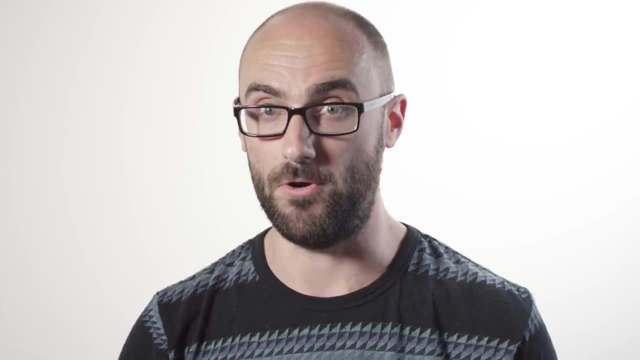 as long as every part of it contains a beginning element, the whole thing describes a new ordinal number, Always. This will be very important later on. It should be noted at this point that if you are ever playing a game of who can name the biggest number, 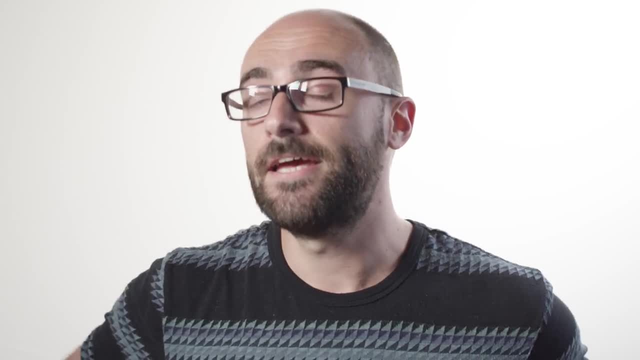 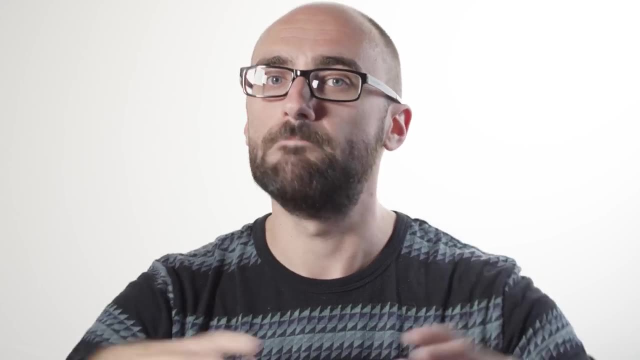 and you're considering saying omega plus 1, you should be careful. Your opponents might require the number you name to be a cardinal. that refers to an amount. These numbers are called cardinals. These numbers refer to the same amount of stuff, just arranged differently. 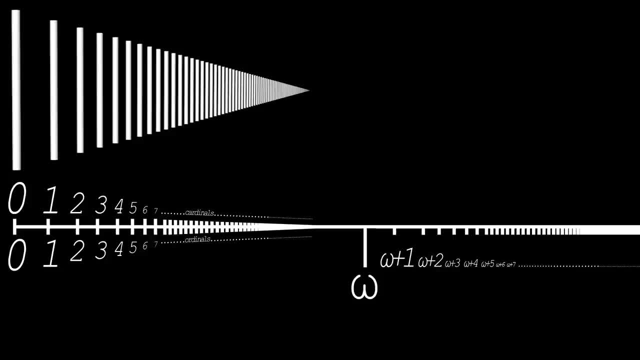 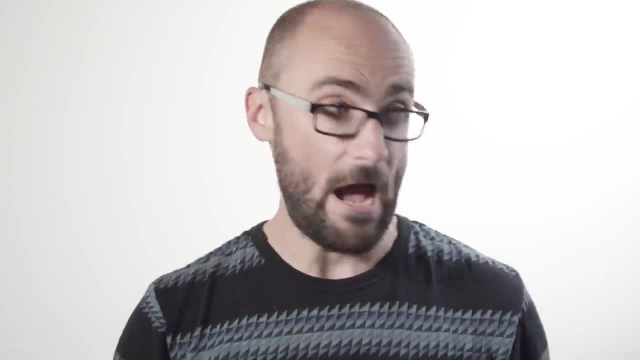 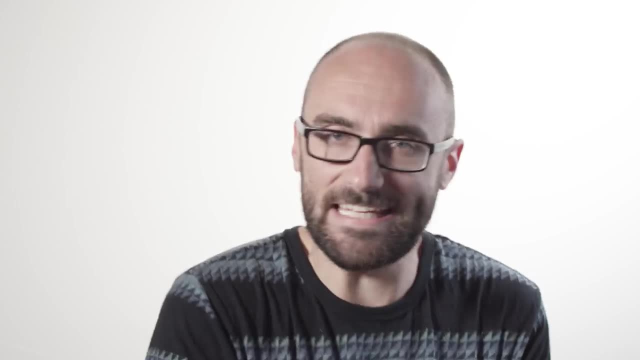 Omega plus 1 isn't bigger than omega, it just comes after omega. But aleph-nol isn't the end. Why? Well, because it can be shown that there are infinities bigger than aleph-nol that literally contain more things. 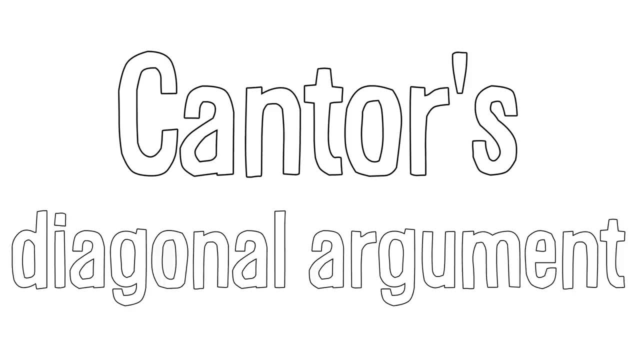 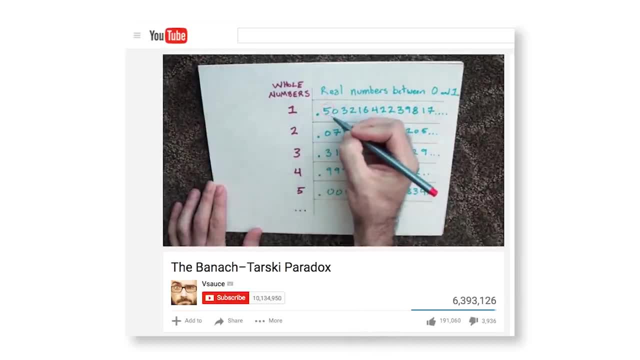 One of the best ways to do this is with Cantor's diagonal argument. In my episode on the Bonok-Tarski paradox, I used it to show that the number of real numbers is larger than the number of natural numbers. But for the purposes of this video, 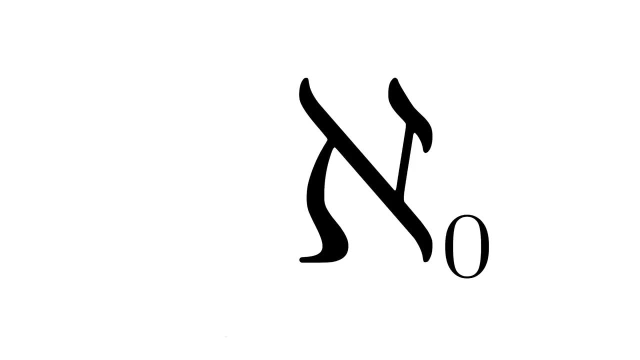 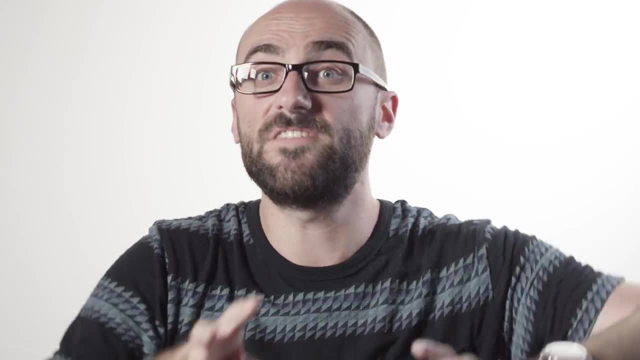 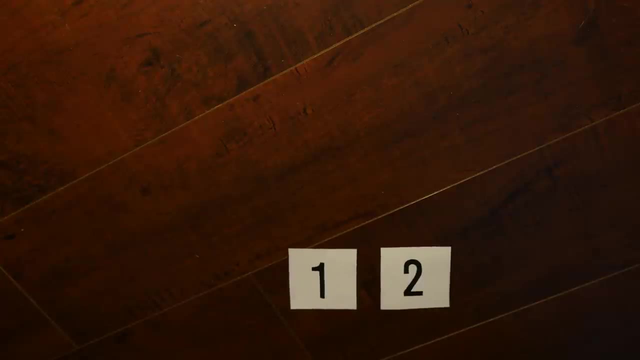 let's focus on another thing bigger than aleph-nol: the power set of aleph-nol. The power set of a set is the set of all the different subsets you can make from, For example, from the set of 1 and 2, I can make a set of nothing. 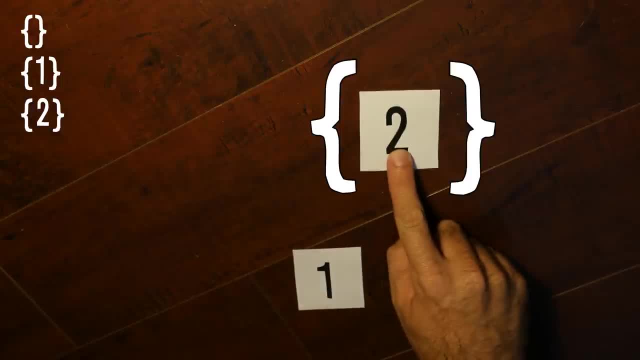 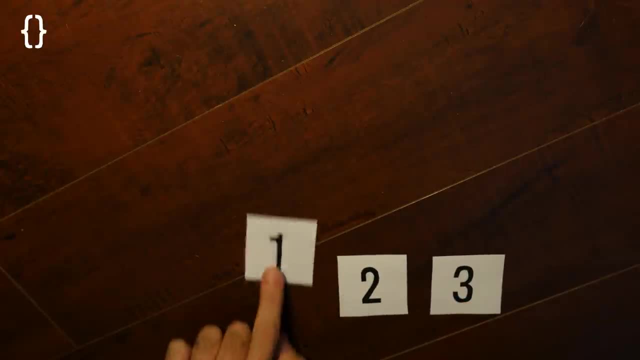 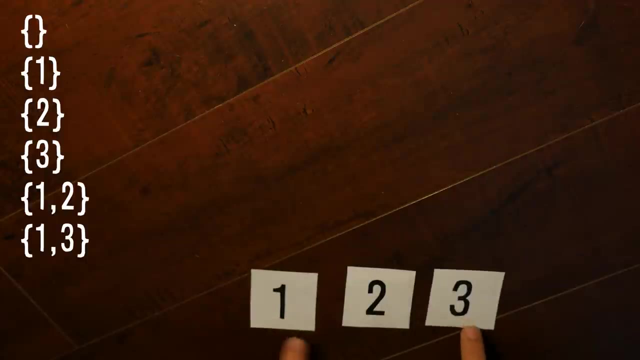 or 1, or 2, or 1 and 2.. The power set of 1,, 2, 3 is the empty set: 1, and 2, and 3, and 1 and 2, and 1 and 3, and 2 and 3, and 1,, 2, 3.. 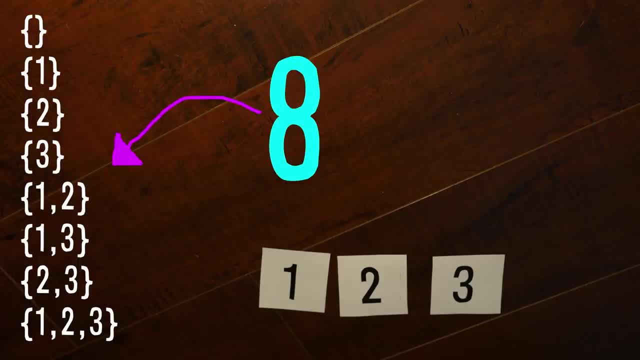 As you can see, a power set contains many more members than the original set. 2 to the power of however many members. the original set had to be exact. So what's the power set of all the naturals? Well, let's see. 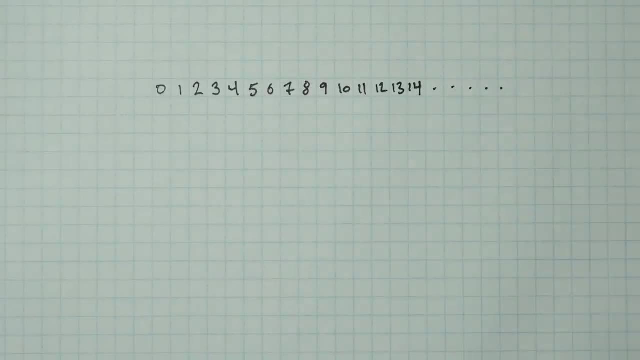 Imagine a list of every natural number. Cool, Now. the subset of all, say, even numbers would look like this: Yes, no, yes, no, yes, no, and so on. The subset of all odd numbers would look like this: 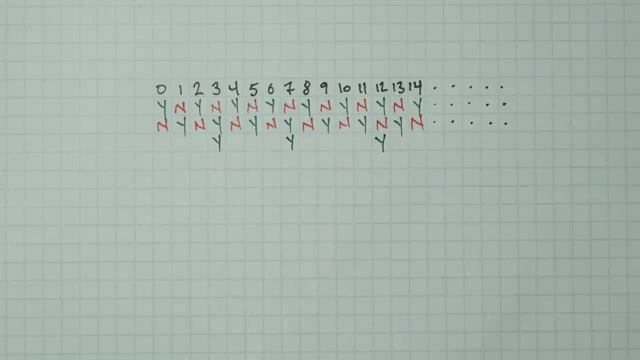 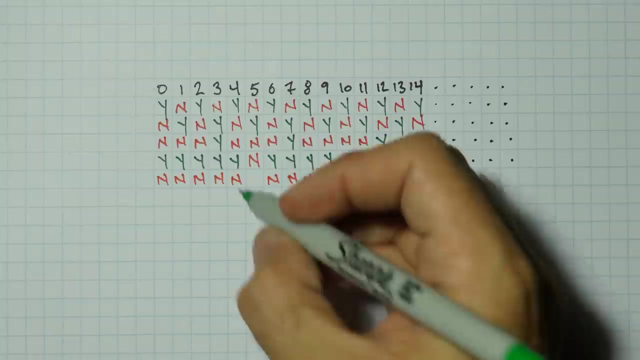 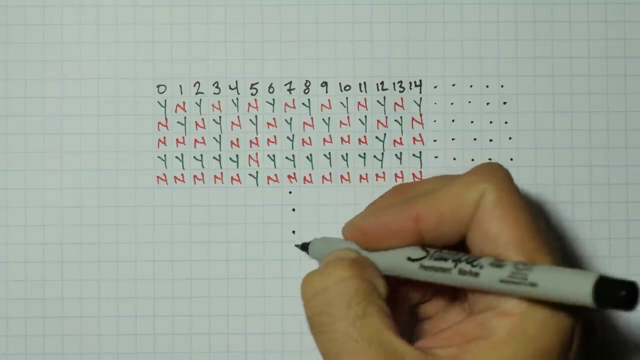 Here's the subset of just 3,, 7,, 8. And 12.. And how about every number except 5?? Or no number except 5?? Obviously, this list of subsets is going to be well infinite, But imagine matching them all one to one with a natural. 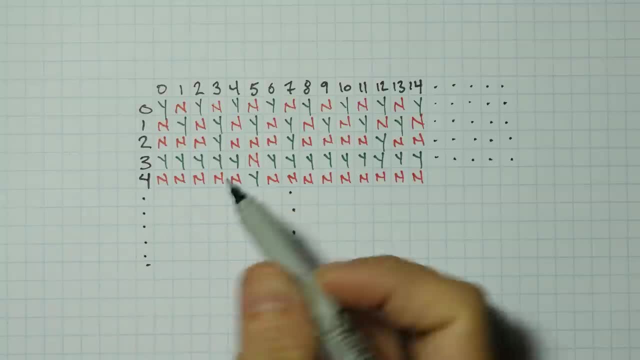 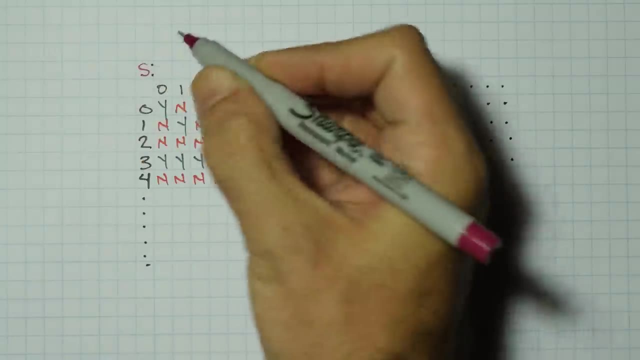 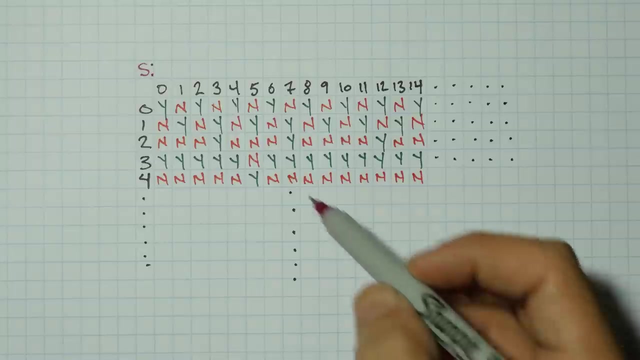 If, even then, there's a way to keep producing new subsets that are clearly not listed anywhere here, we will know that we've got a set with more members than there are natural numbers, A bigger infinity than aleph null. The way to do this is to start up here, in the first subset. 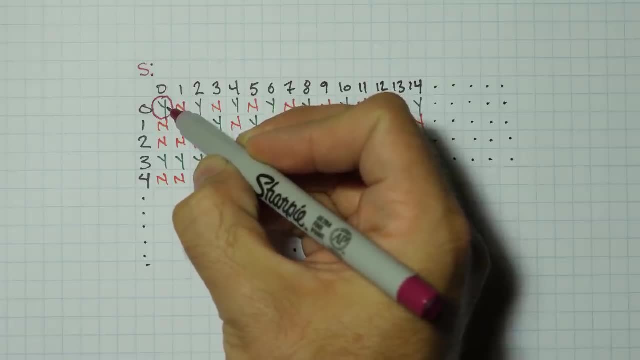 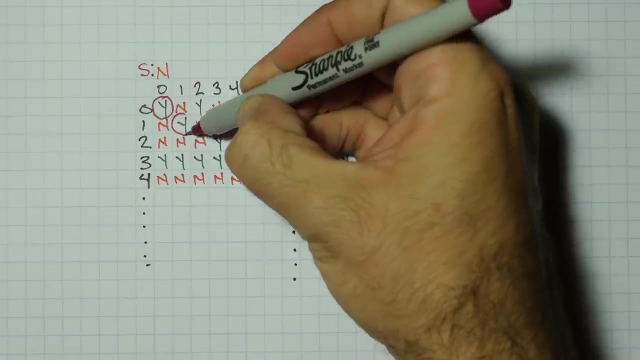 and just do the opposite of what we see. 0 is a member of this one, so our new set will not contain 0.. Next move diagonally down to 1's membership in the second subset. 1 is a member of it, so it will not be in our new set. 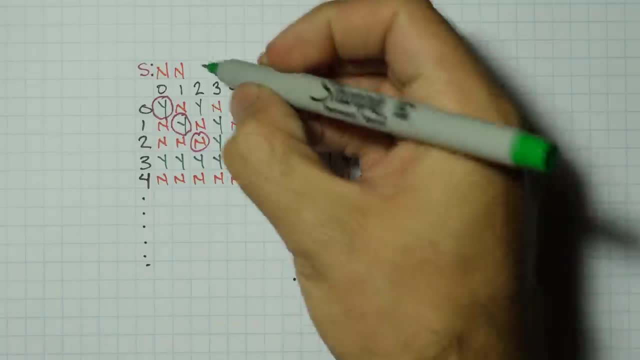 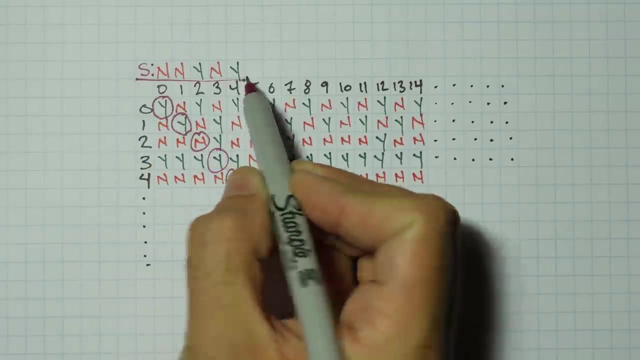 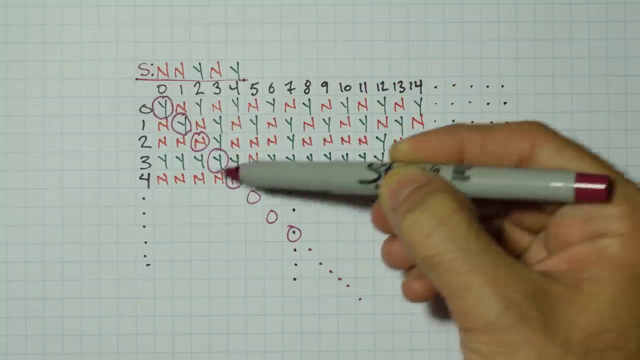 2 is not in the third subset, so it will be in ours, and so on. As you can see, we are describing a subset that will be, by definition, different in at least one way from every single other subset on this aleph null-sized list. 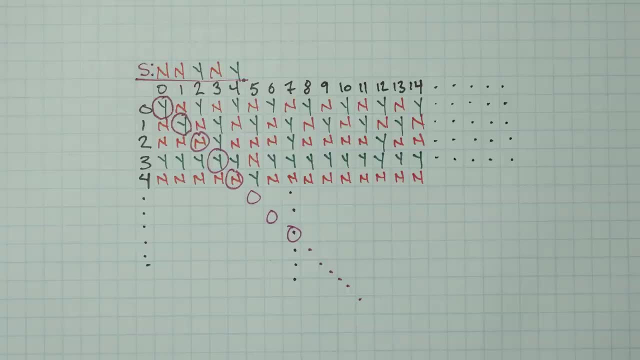 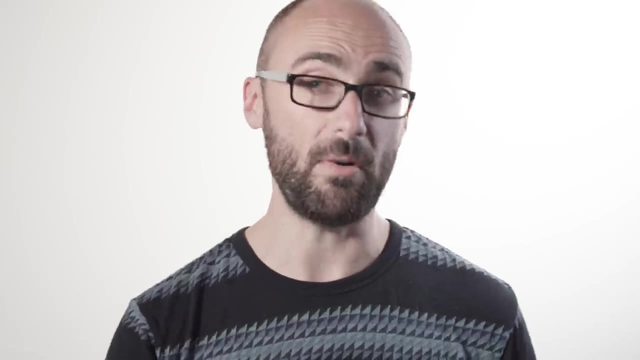 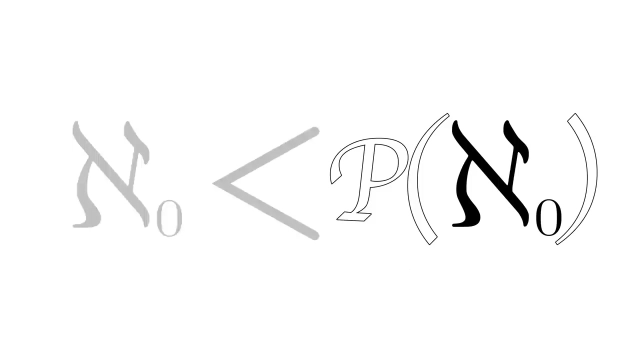 Even if we put this new subset back in, diagonalization can still be done. The power set of the naturals will always resist a one-to-one correspondence with the naturals. It's an infinity bigger than aleph null. Repeated applications of power set will produce sets. 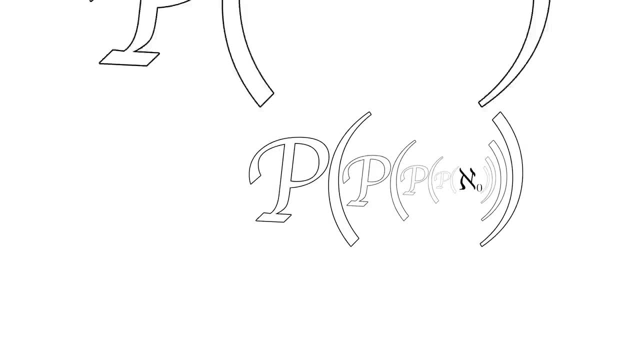 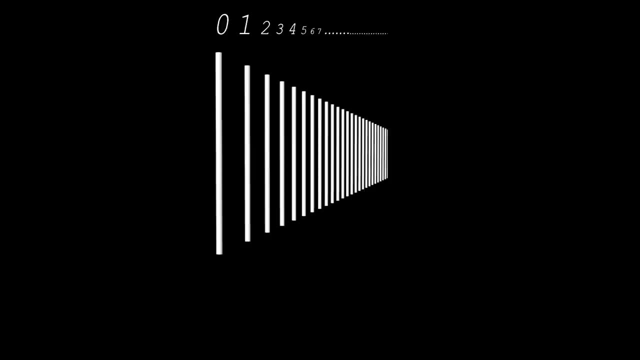 that can't be put into one-to-one correspondence with the last. so it's a great way to quickly produce bigger and bigger infinities. The point is there are more cardinals after aleph null. Let's try to reach them. 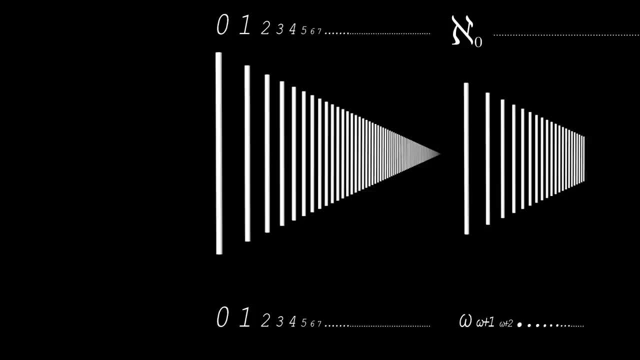 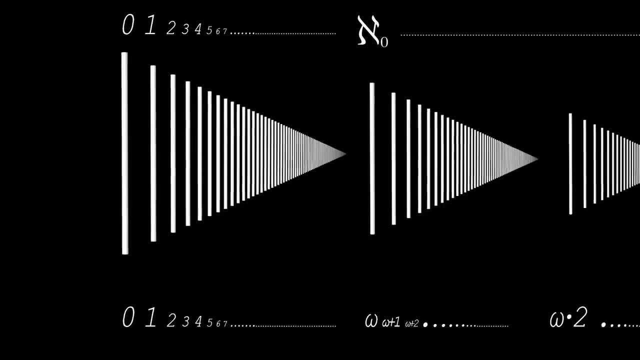 Now remember that after omega, ordinals split and these numbers are no longer cardinals, They don't refer to a greater amount than the last cardinal we reached, but maybe they can take us to one. Wait, what are we doing? 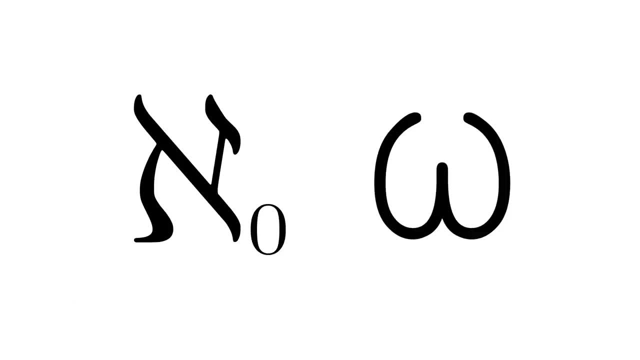 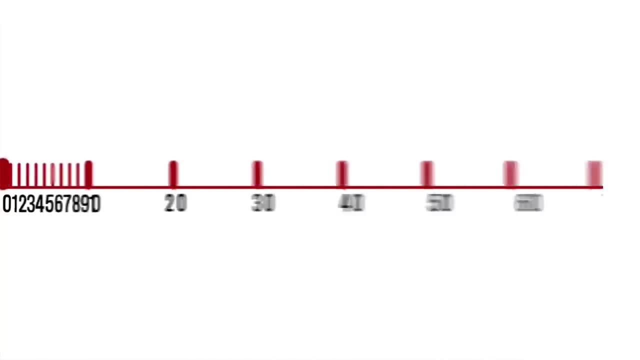 Aleph, null, Omega, Come on, we've been using these numbers like there's no problem. But if at any point down here, you can always add one, Always, Can we really talk about it, This endless process as a totality, and then follow it with something? 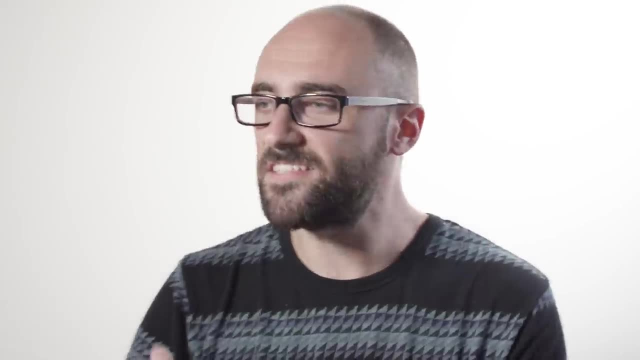 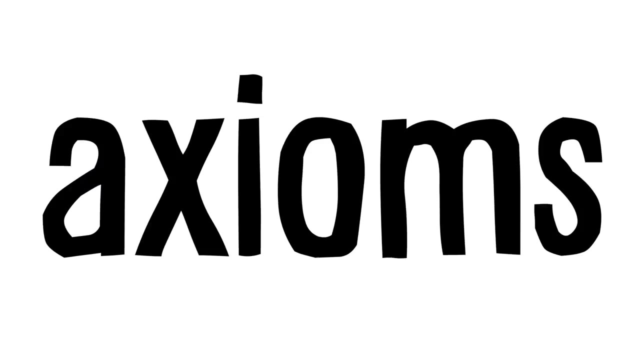 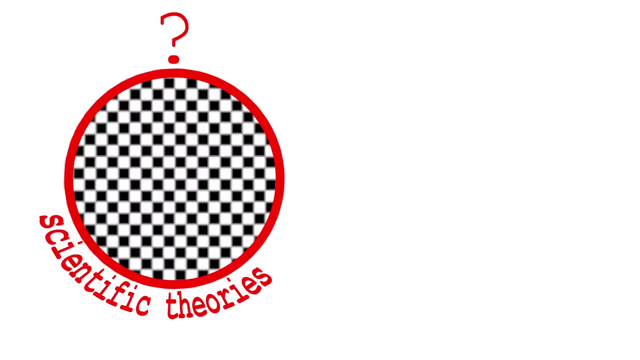 Of course we can. This is math, not science. The things we assume to be true in math are called axioms, and an axiom we come up with isn't more likely to be true if it better explains or predicts what we observe. Instead, it's true because we say it is. 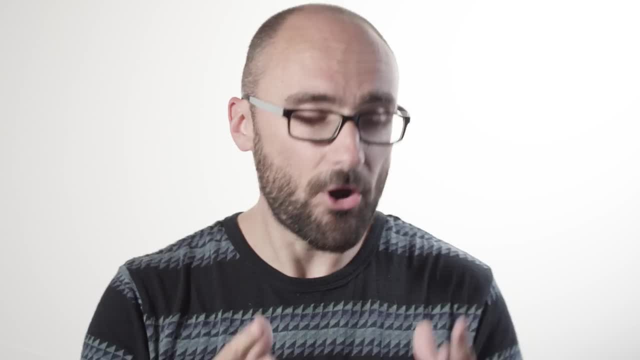 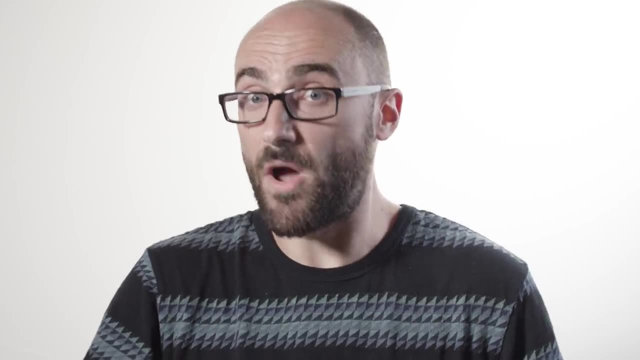 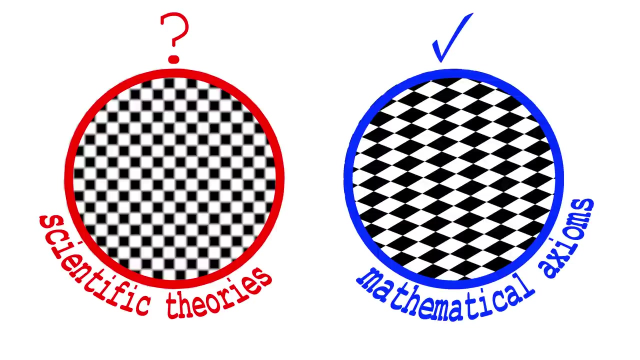 Its consequences just become what we observe. We are not fitting our theories to some physical universe whose behavior and underlying laws would be the same whether we were here or not. We are creating this universe ourselves If the axioms we declare to be true lead us to contradictions or paradoxes. 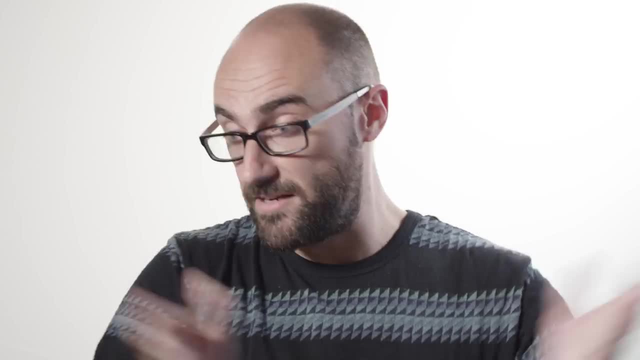 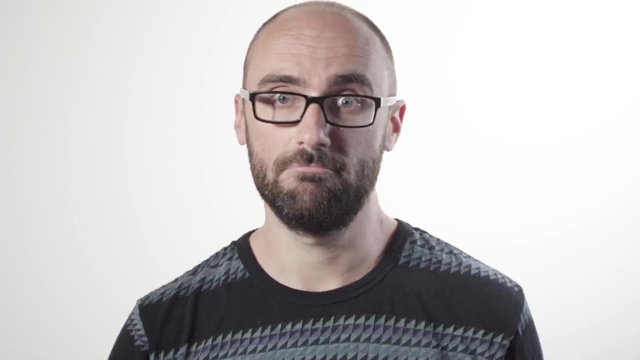 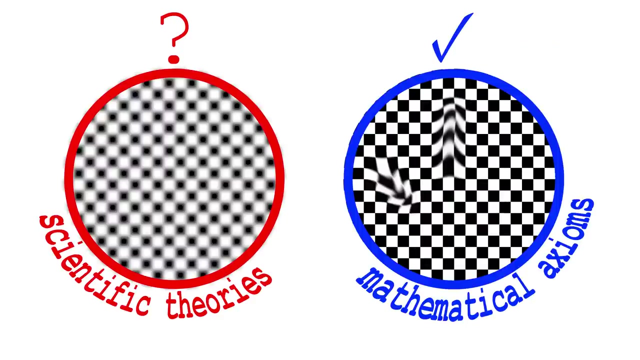 we can go back and tweak them or just abandon them altogether, or we can just refuse to allow ourselves to do the things we want to do. We refuse to allow ourselves to do the things that cause the paradoxes. That's it. What's fascinating, though, is that, in making sure the axioms we accept don't lead to problems, 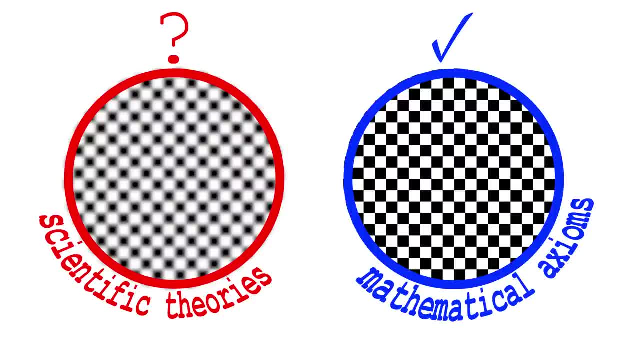 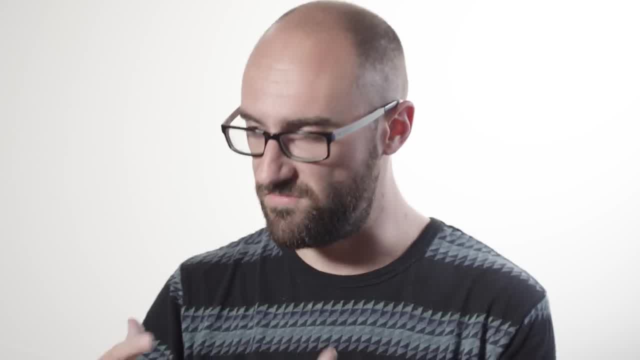 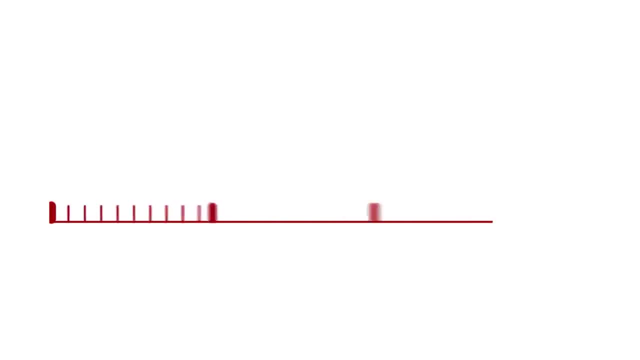 we've made math into something that is, as the saying goes, unreasonably effective in the natural sciences. So to what extent we're inventing all of this or discovering it, it's hard to say. All we have to do to get omega is say: 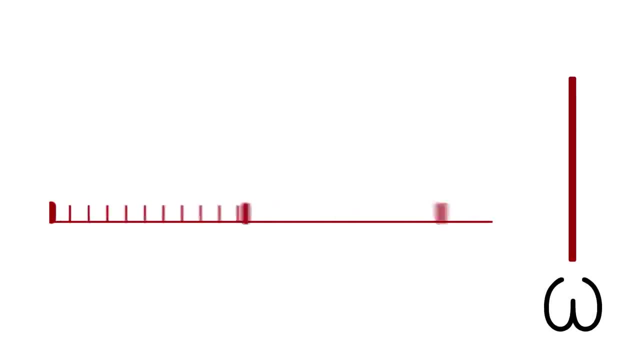 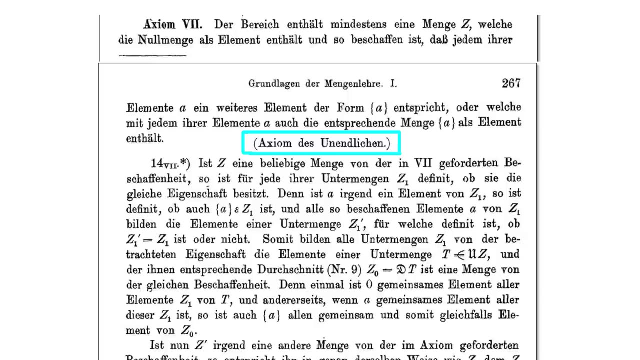 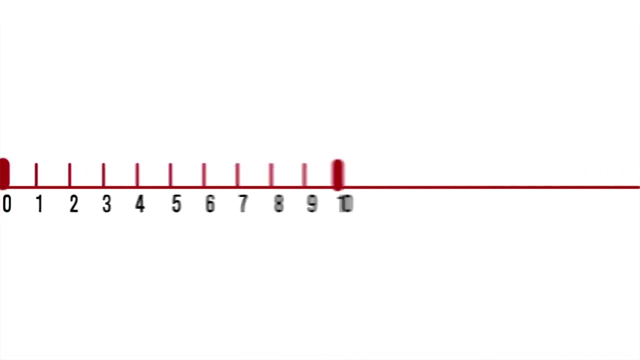 let there be omega and it will be good. That's what Ernest Zermelo did in 1908 when he included the axiom of infinity in his list of axioms for doing stuff in math. The axiom of infinity is simply the declaration that one infinite set exists. 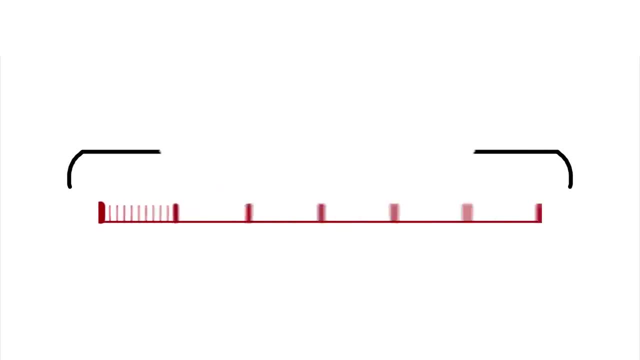 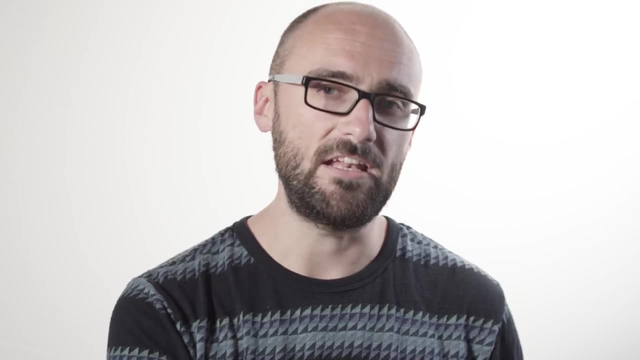 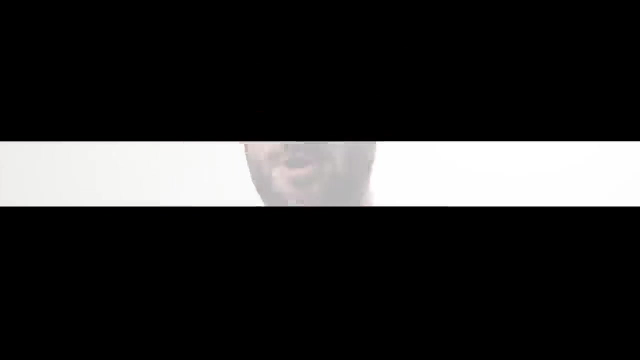 The set of all natural numbers. If you refuse to accept it, that's fine. That makes you a finitist one who believes only finite things exist. But if you accept it, as most mathematicians do, you can go pretty far. 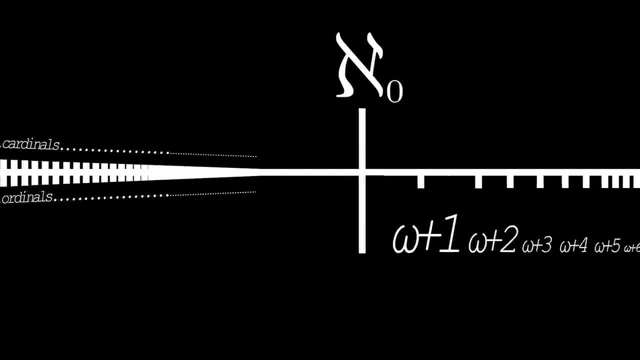 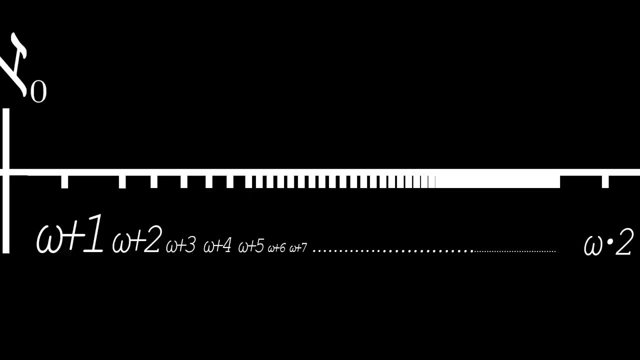 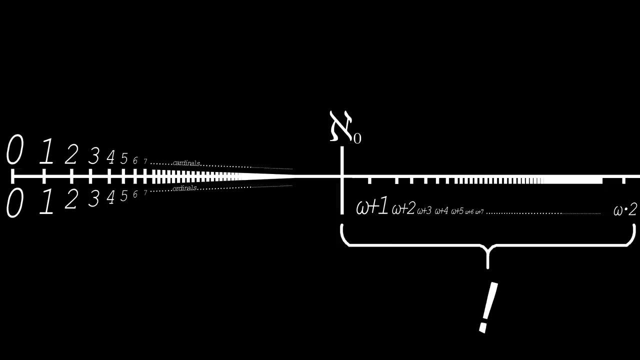 Past these and through these, Eventually we get to omega plus omega, except we've reached another ceiling. Going all the way out to omega plus omega would be to create another infinite set, And the axiom of infinity only guarantees that this one exists. 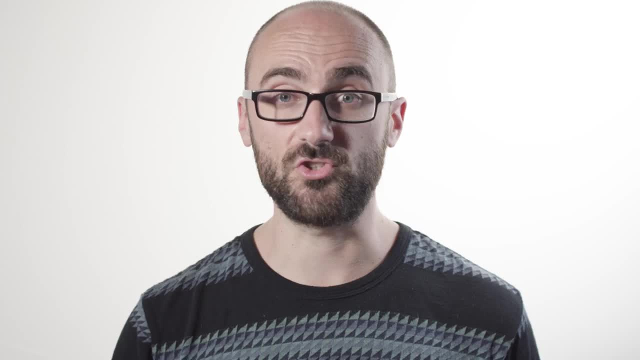 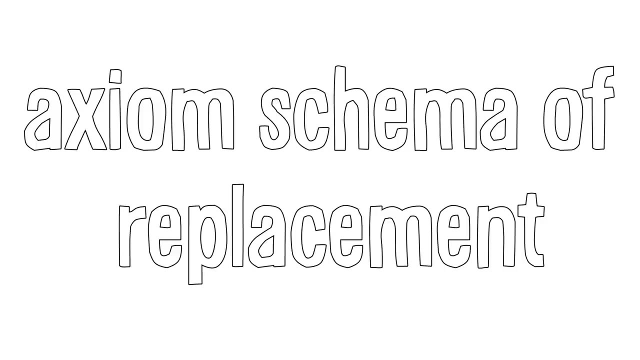 Are we going to have to add a new axiom every time we describe Aleph Noll Moore numbers? No, The axiom of replacement can help us here. This assumption states that if you take a set like, say, the set of all natural numbers, 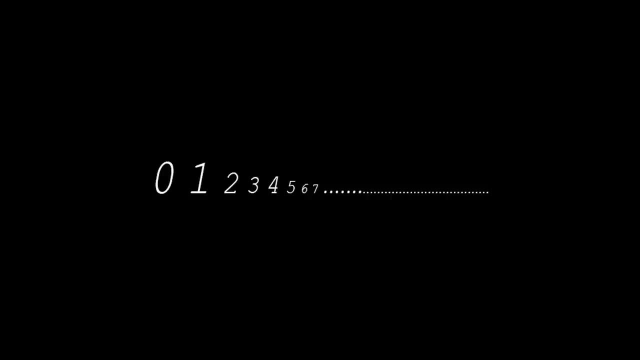 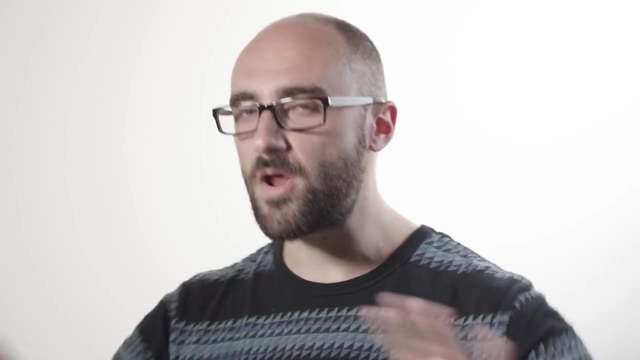 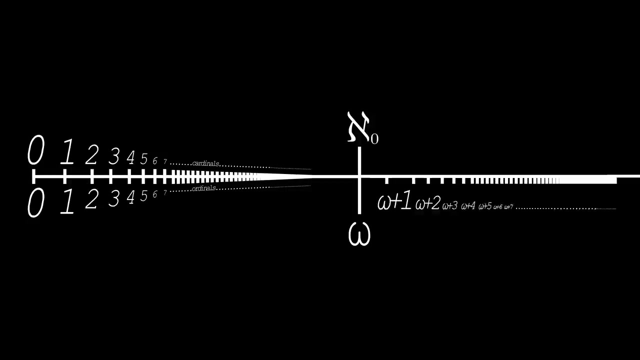 and replace each element with something else, like, say, bananas. what you're left with is also a set. That sounds simple, but it's incredibly useful. Try this: Take every ordinal up to omega and then, instead of bananas, put omega plus in front of each. 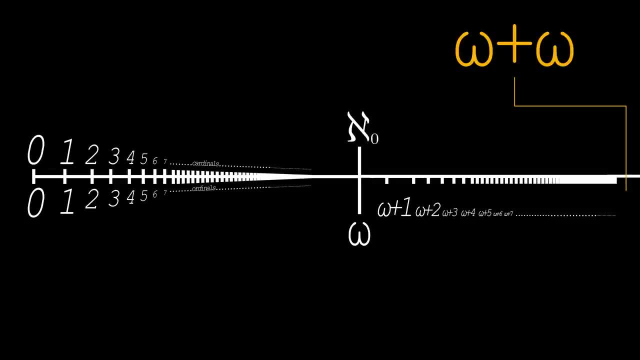 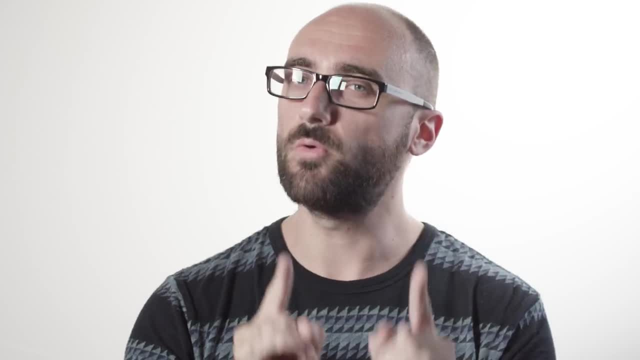 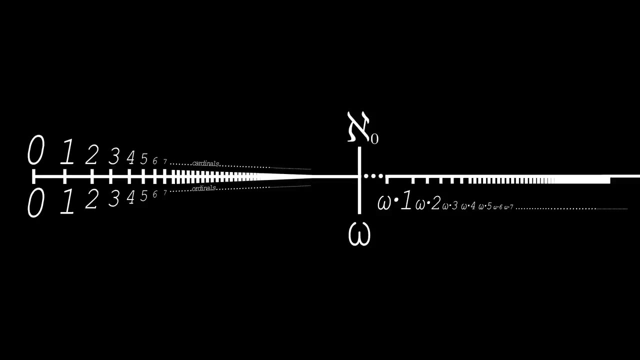 Now we've reached omega plus omega or omega times two. Using replacement, we can make jumps of any size we want, so long as we only use numbers we've already achieved. We can replace every ordinal up to omega with omega times. it. 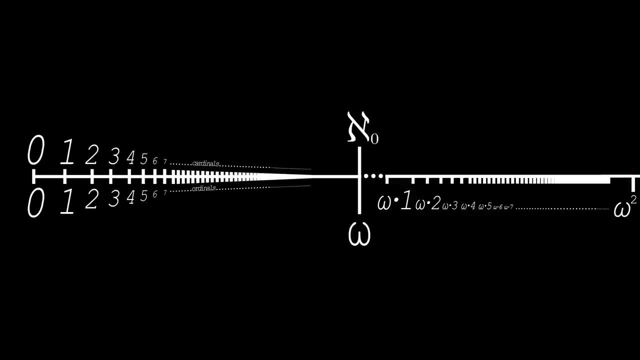 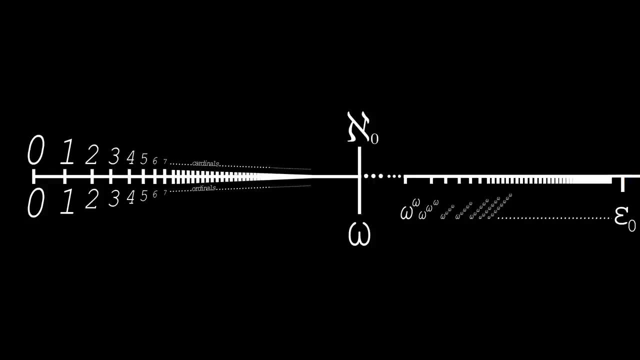 No problem, This is just called epsilon naught, and we continue from here. But now think about all of these, all of these ordinals, all the different ways to arrange aleph-null things. Well, these are well-ordered. 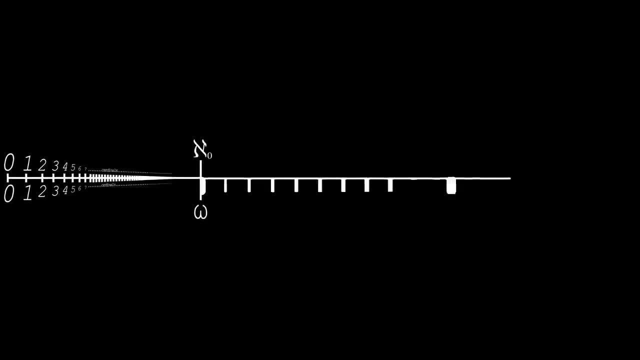 so they have an order type, some ordinal, that comes after all of them. In this case, that ordinal is called omega one. Now, because by definition omega one comes after every single order type of aleph-null things, it must describe an arrangement of literally more stuff than the last aleph. 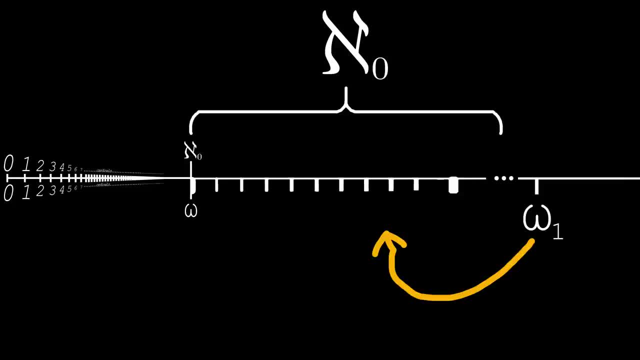 I mean, if it didn't it would be somewhere in here, But it's not The cardinal number describing the amount of things used to make an arrangement with order type omega one is aleph-one. It's not known where the power set of the naturals falls on this line. 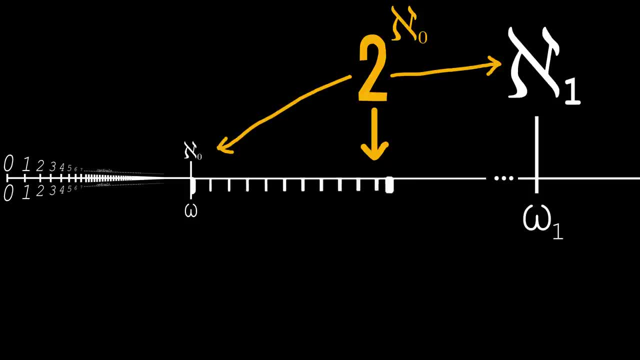 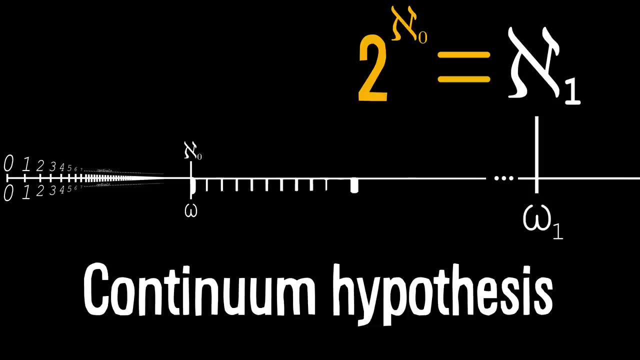 It can't be between these cardinals because, well, there aren't cardinals between them. It could be equal to aleph-one. That belief is called the continuum hypothesis, But it could also be larger. We just don't know. 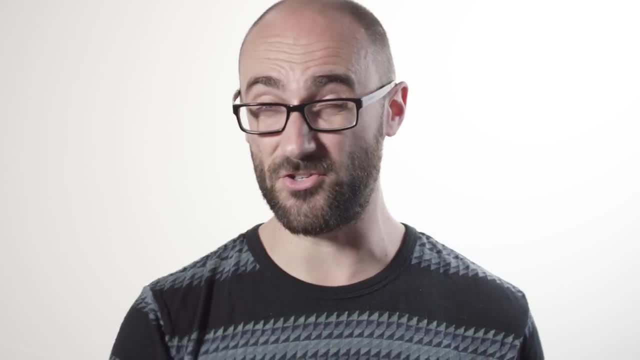 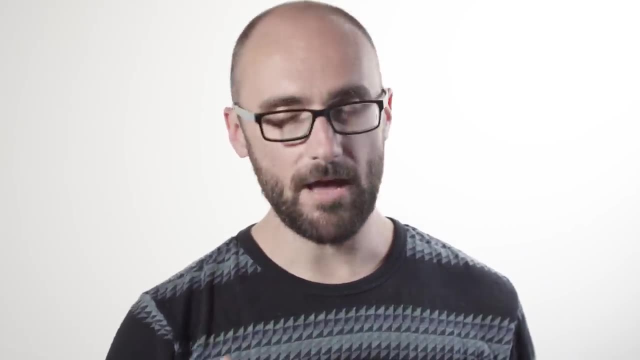 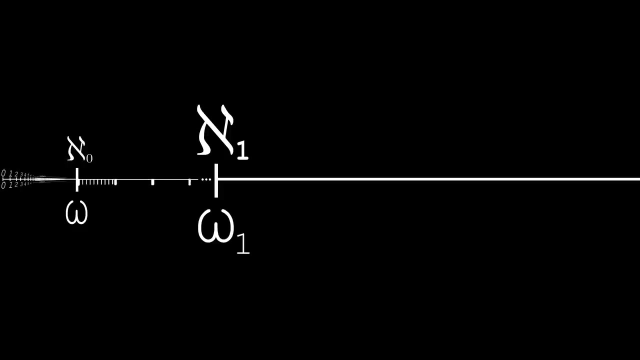 The continuum hypothesis, by the way, is probably the greatest unanswered question in this entire subject, And today, in this video, I will not be solving it, but I will be going higher and higher, to bigger and bigger infinities. Now, using the replacement axiom. we can take any ordinal we already reached, like, say, omega, and jump from aleph to aleph all the way out to aleph-omega Or heck. why not use a bigger ordinal like omega-squared to construct aleph-omega-squared? 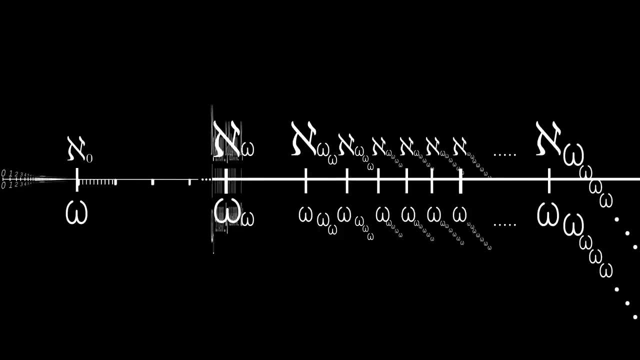 Aleph-omega-omega-omega-omega-omega-omega-omega. Our notation only allows me to add countably many omegas here, but replacement doesn't care about whether or not I have a way to write the numbers it reaches. 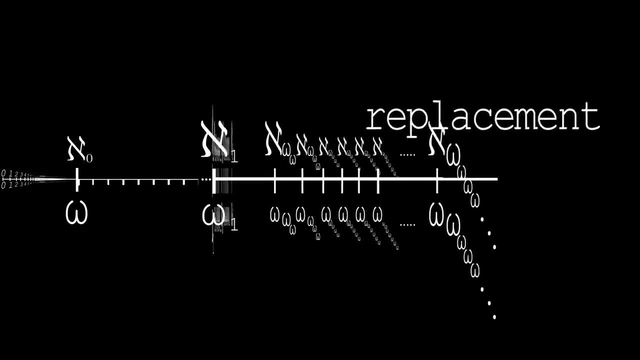 Wherever I land will be a place of even bigger numbers, allowing me to make even bigger and bigger numbers and more numerous jumps than before. The whole thing is a wildly accelerating feedback loop of embiggening. We can keep going like this. 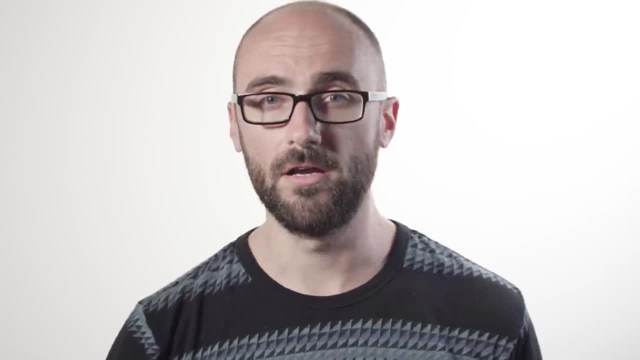 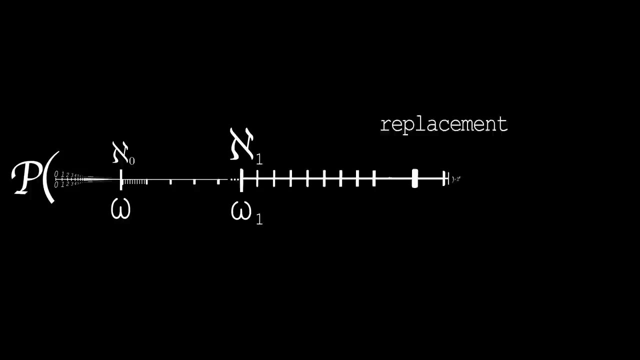 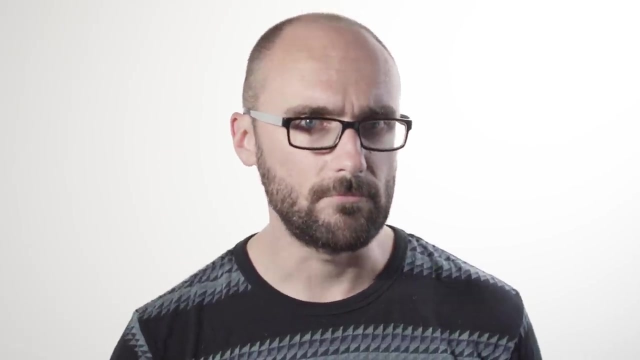 reaching bigger and bigger infinities from below. Replacement and repeated power sets, which may or may not line up with the alephs, can keep our climb going forever. So clearly, there's nothing beyond them, Right? Not so fast. 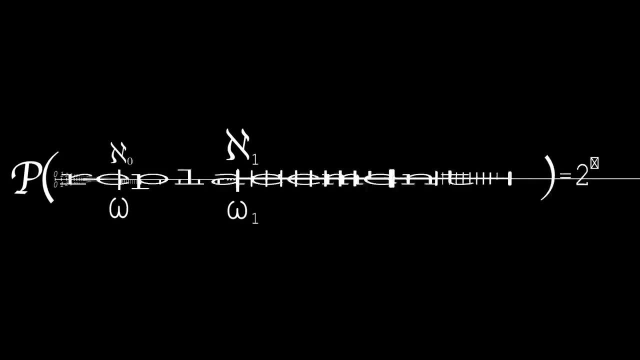 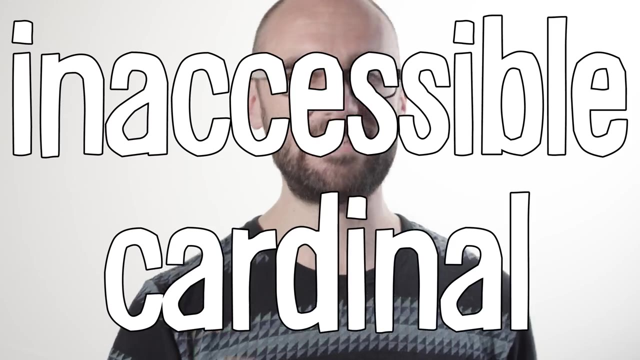 That's what we said about getting past the finite to omega. Why not accept as an axiom that there exists some next number so big? no amount of replacement or power setting on anything smaller could ever get you there. Such a number is called an inaccessible cardinal. 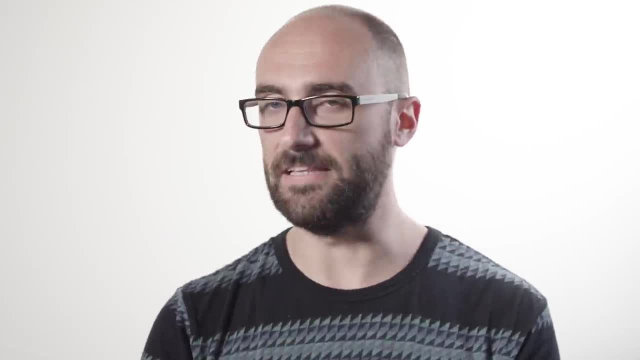 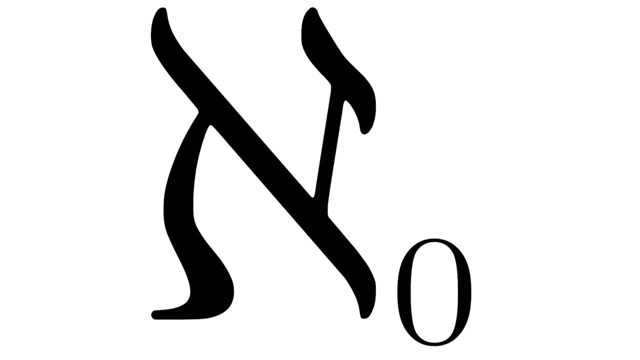 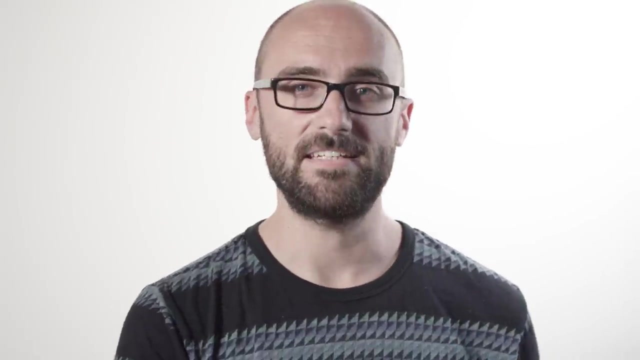 because you can't reach it from below. Now, interestingly, within the numbers we've already reached, a shadow of such a number can be found: Aleph null. You can't reach this number from below either. All numbers less than it are finite. 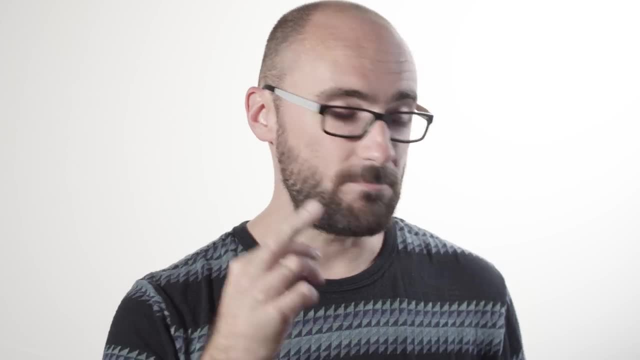 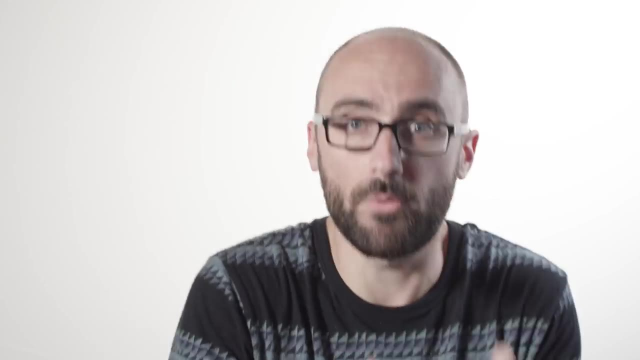 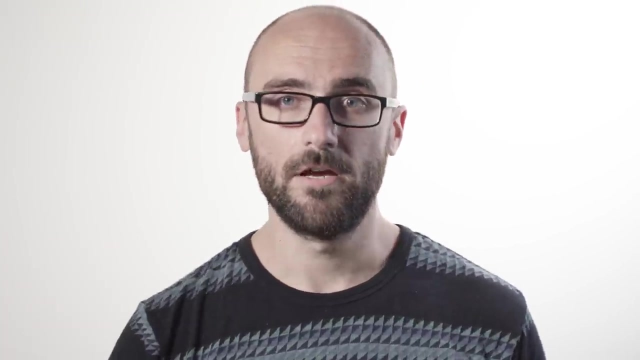 And a finite number of finite numbers can't be added, multiplied, exponentiated, replaced with finite jumps, a finite number of times, or even power set a finite number of times to give you anything but another finite amount. Sure, the power set of a millenillion to a googolplex, to a googolplex to a googolplex. 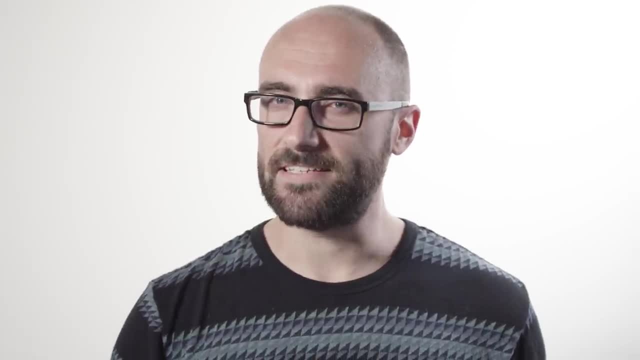 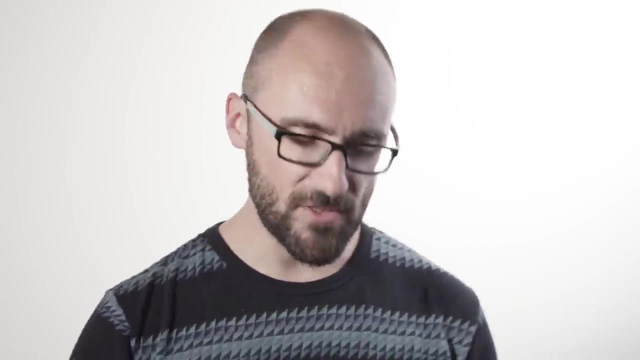 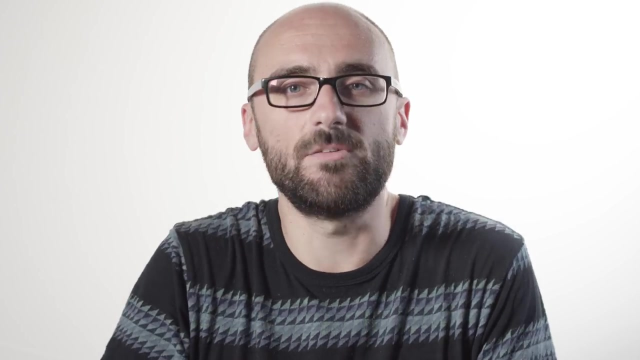 is really big, but it's still just finite, Not even close to aleph null, the first, smallest infinity. For this reason, aleph null is often considered an inaccessible number. Some authors don't do this, though. saying an inaccessible must also be uncountable. 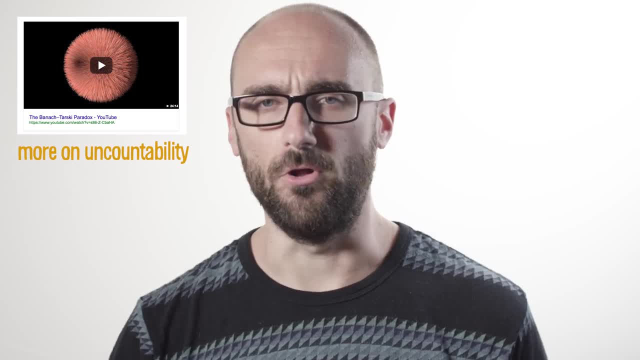 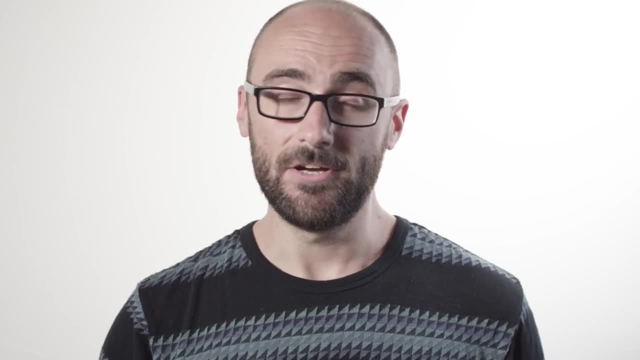 which, okay, makes sense. I mean, we've already accessed aleph null, But remember, the only way we could is by straight up declaring its existence axiomatically. We will have to do the same for inaccessible cardinals. It's really hard to get across. 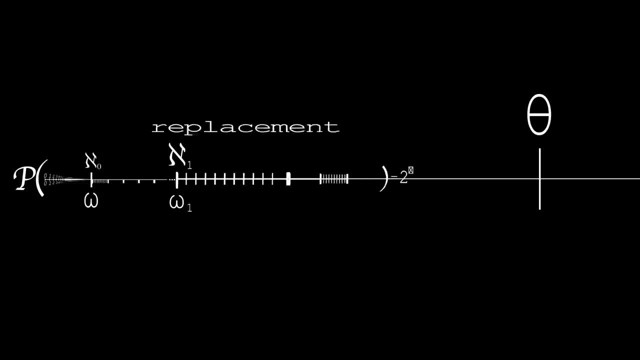 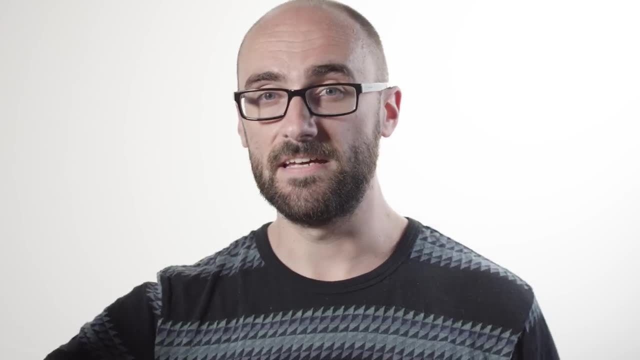 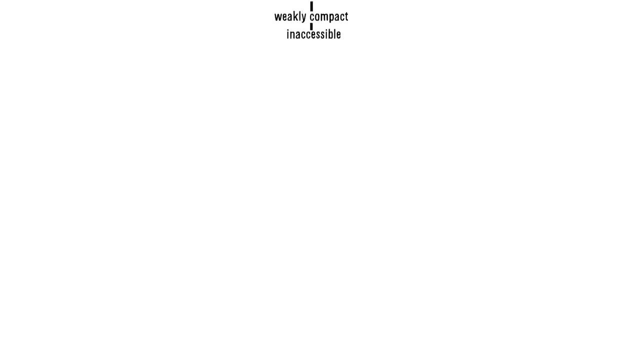 just how unfathomable the size of an inaccessible cardinal is. I'll just leave it at this. The conceptual jump from nothing to the first infinity is like the jump from the first infinity to an inaccessible Set. theorists have described numbers bigger than inaccessibles. 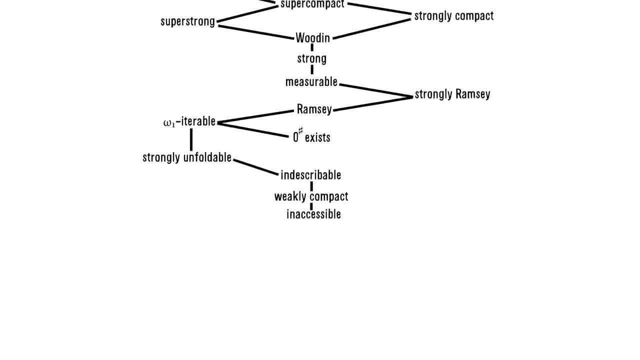 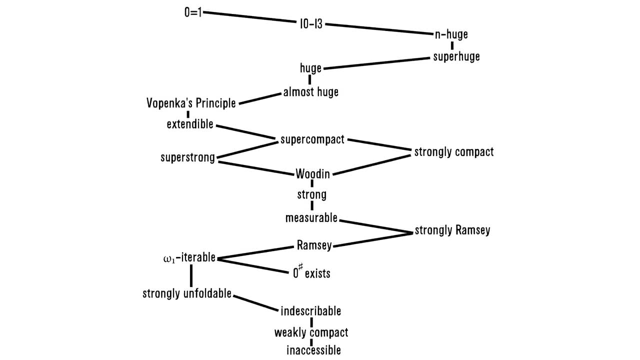 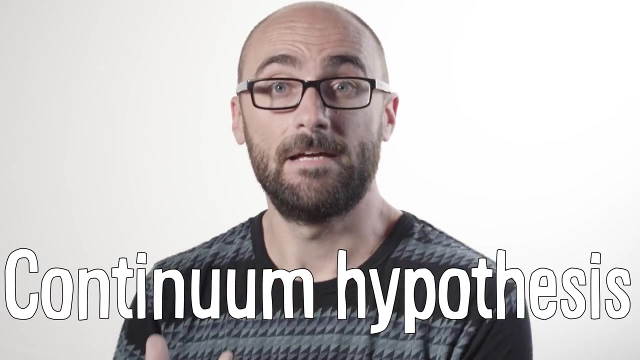 each one requiring a new large, cardinal axiom asserting its existence, expanding the height of our universe of numbers? Will there ever come a point where we devise an axiom implying the existence of so many things that it implies contradictory things? Will we someday answer the Continuum Hypothesis? 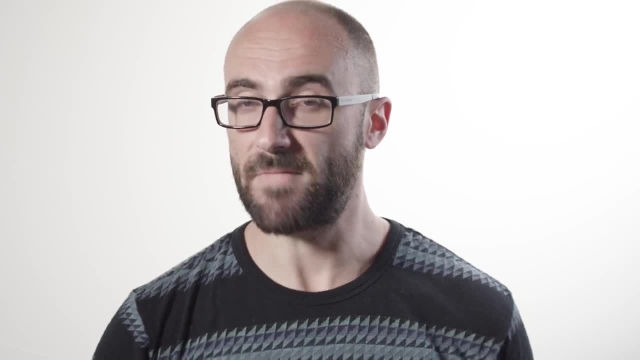 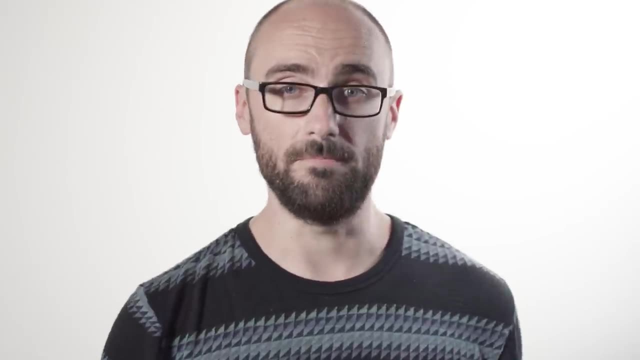 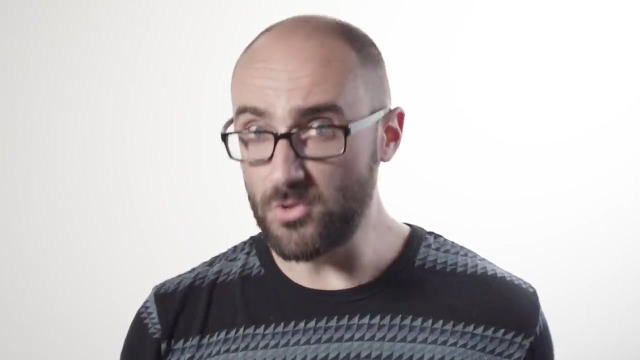 Maybe not, but there are promising directions. And until then, the amazing fact remains that many of these infinities- perhaps all of them- are so big it's not exactly clear whether they even truly exist or could be shown to in the physical universe. 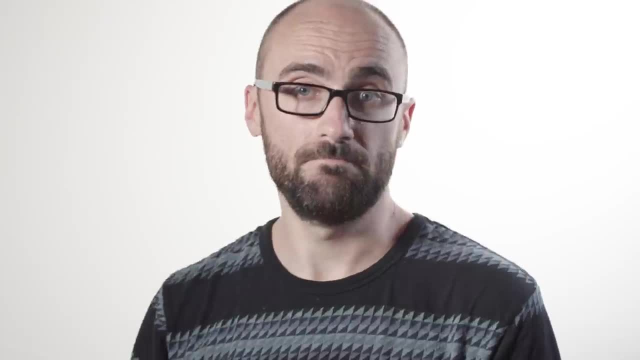 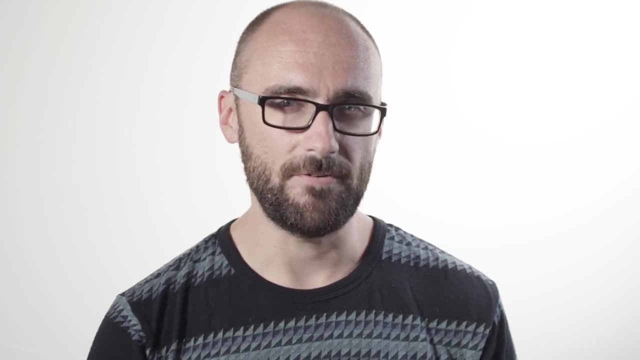 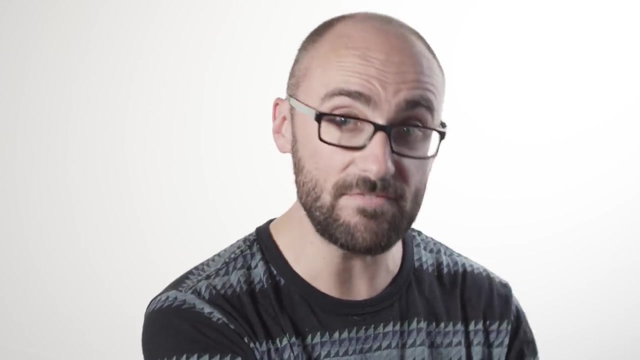 If they do, if one day physics finds a use for them, that's great, But if not, that's great too. That would mean that we have with this brain a tiny thing, a septillion times smaller than the tiny planet it lives on.